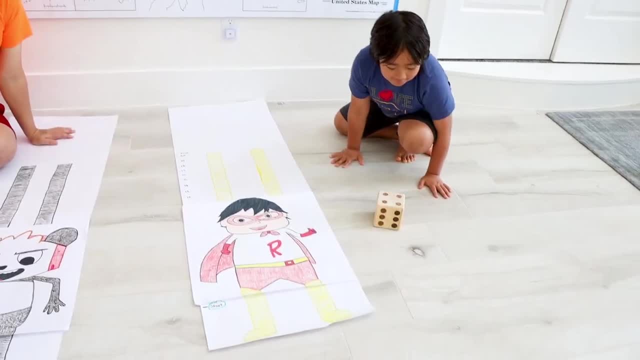 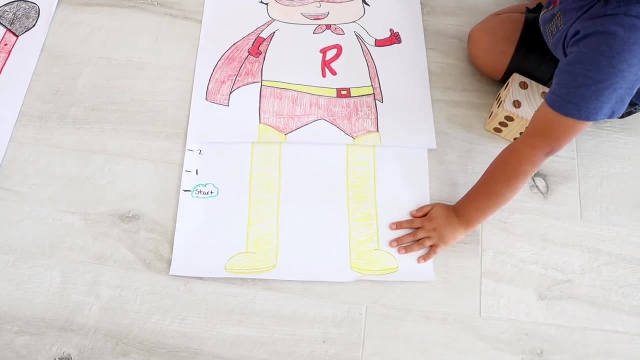 Let's see how tall I can get Red Titan. It's pretty short right now. He's four. Oh nice, Okay. so move up by four. Okay, Two, three, four, Boom, No. So that means Red Titan's taller than Combo. 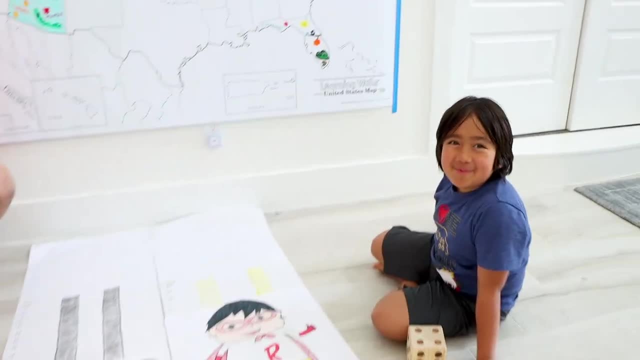 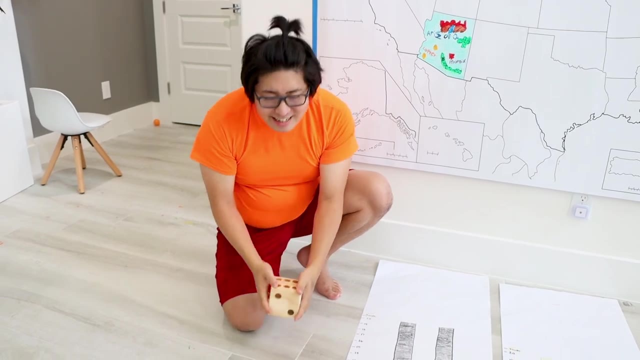 Look at this: He's tall Titan. It's very weird. It is okay, It's my turn. Combo's drinking lots of milk, So he's going to get taller. All right, Three, two, one, What, Uh six? 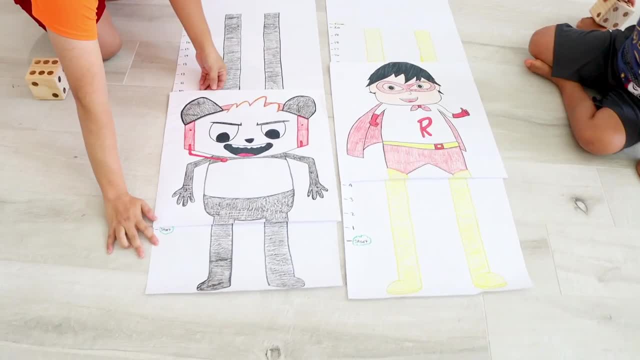 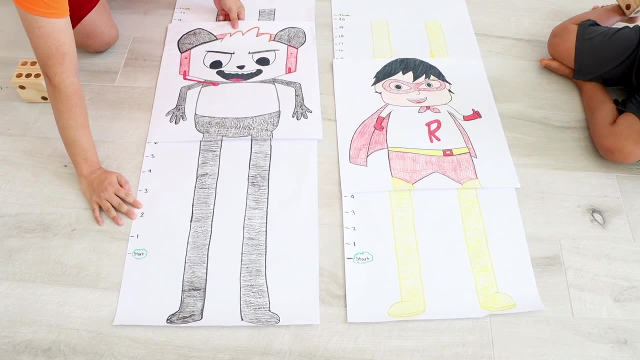 But apparently Combo drinks a lot of milk. Oh yeah, a lot of milk. He grows faster than himself. Boom Boom, Two, three, four, five, six, Whoa Combo. Yeah, he can be a basketball player. 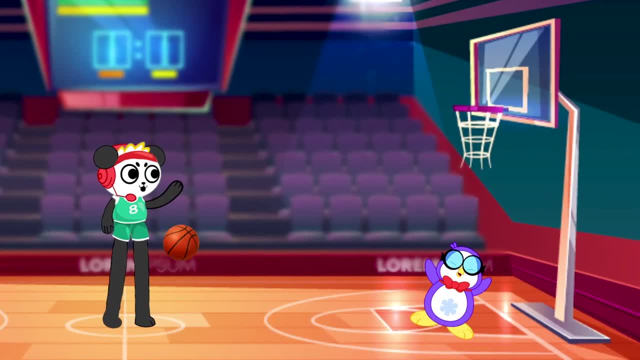 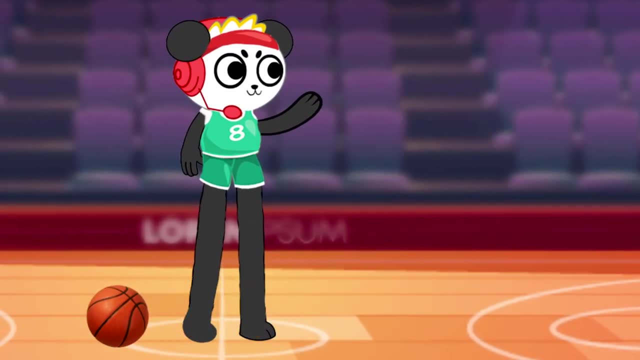 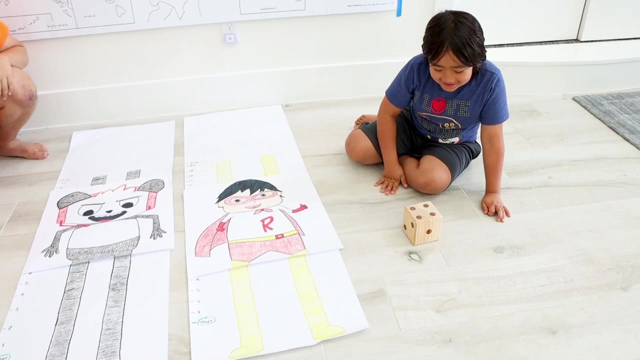 Look at this: Yeah, I wish I had that leg. Oh, I'm game, Oh, no, Okay, now I'm going to go. maybe Red Titan drink a lot of milk. Four again: Oh yeah, that's pretty good. 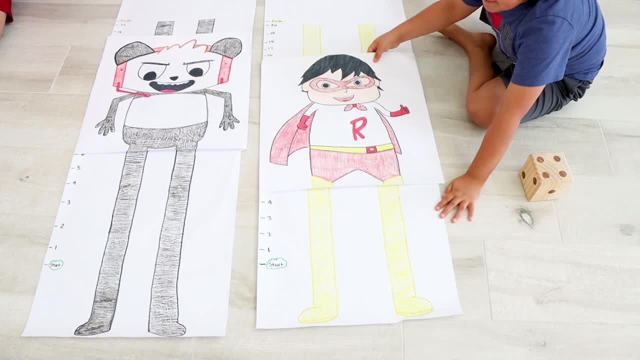 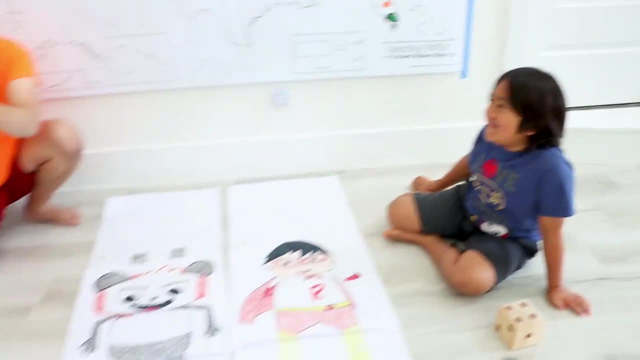 That's pretty good. All right, very consistent. You got four last time, You got four this time too. Now I'm very tall Man, Man Ready, I'm going to spin it a different way. Woo, What Three. 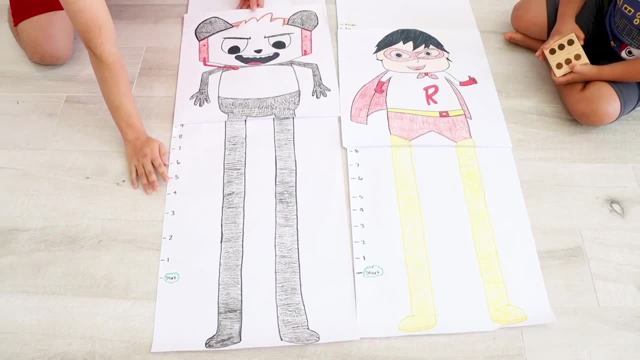 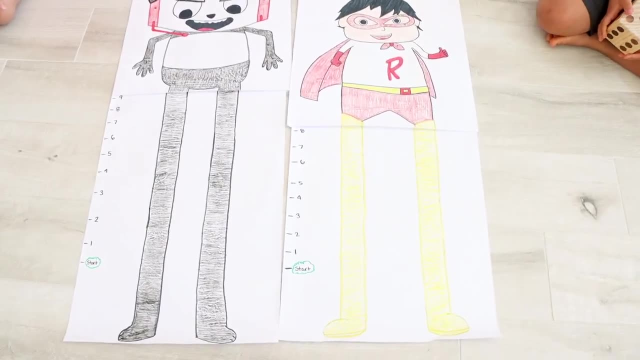 Five, one, two, three Man Combo Still growing. So right now Red Titan is looking like he's a teenager. Yeah, What does he look like when he's 20? I'm ready. Okay, it's my turn. 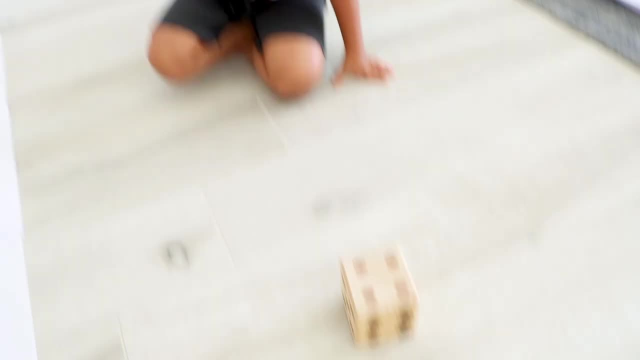 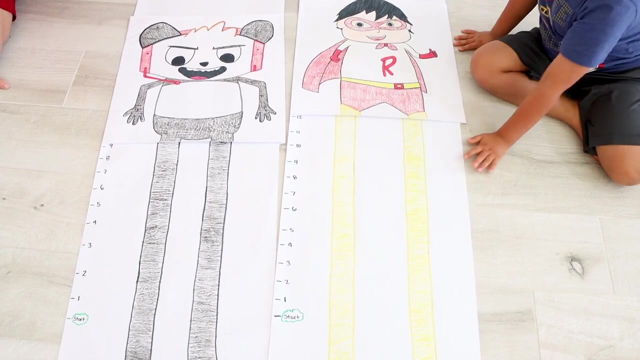 I'm going to spin it. Whoa, I got four. again You're getting four. I keep getting four, Mm-hmm. Okay, One, two, three, four. Oh man, he's so tall. Ugh, Red Titan's looking down on us Combo. 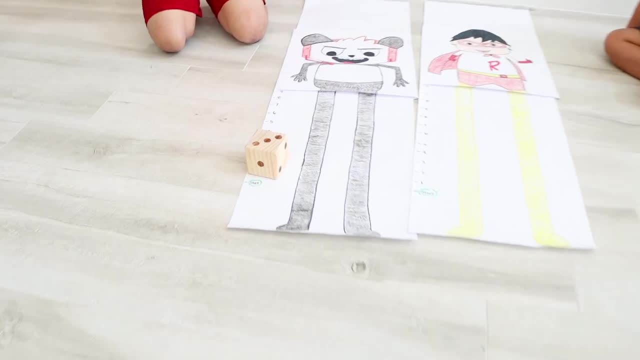 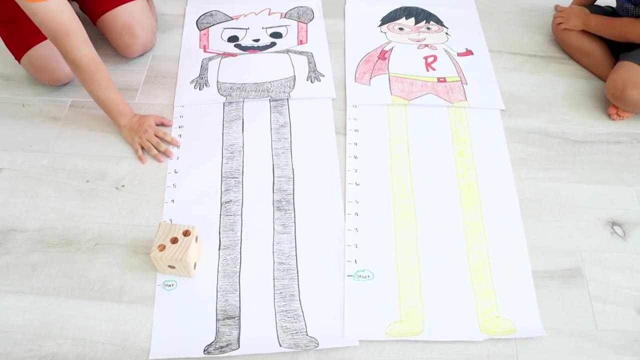 I'll show you. There you go, Woo, Oh, three again. What if I just get four again? One, two, three. Oh, we're the same height. Oh, One, 12 versus 12.. Who's going to get 20?? 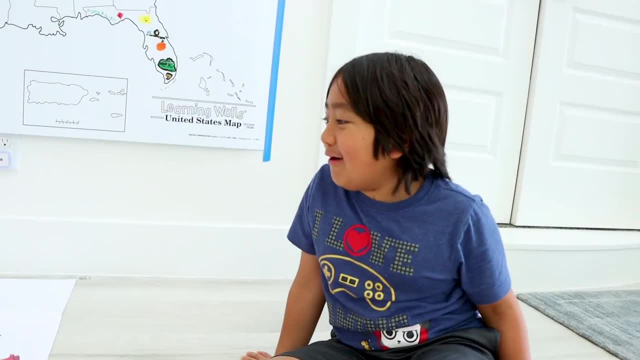 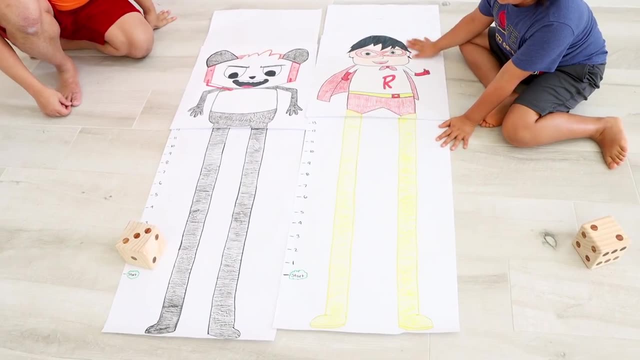 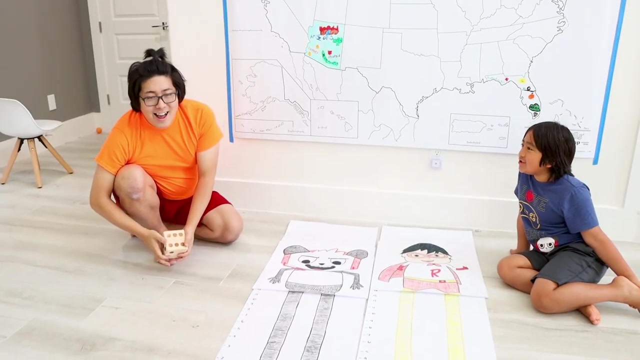 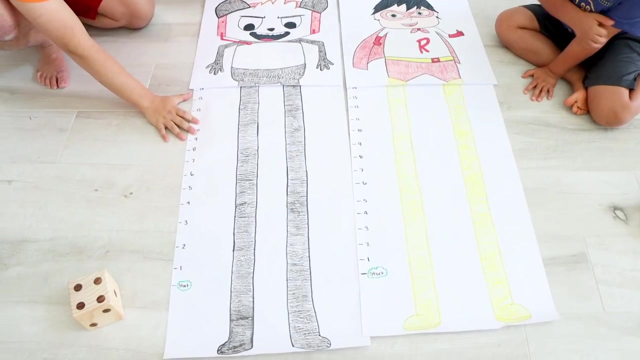 Me, Me, Oh, oh, oh two. I only have 14, but I'm tall. Yes, This is my time to shine. Daddy's not a teenager. And now Combo is very tall. One, two, three, four. 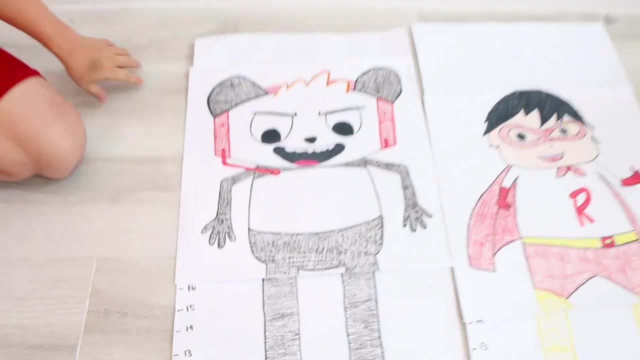 You're so tall, See, he's so tall. That's why he's looking down. Oh my gosh, I'm so tall, I'm scared. So Combo is 16 years old and Red Titan is 14 years old. 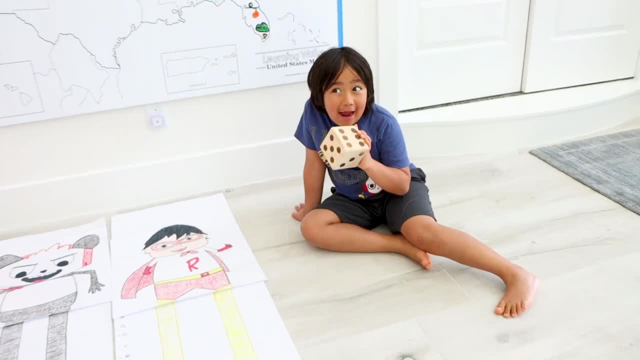 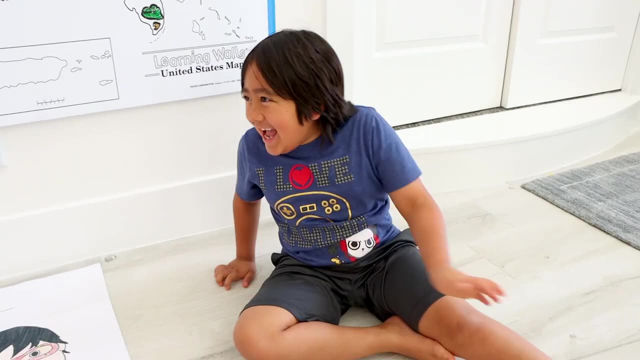 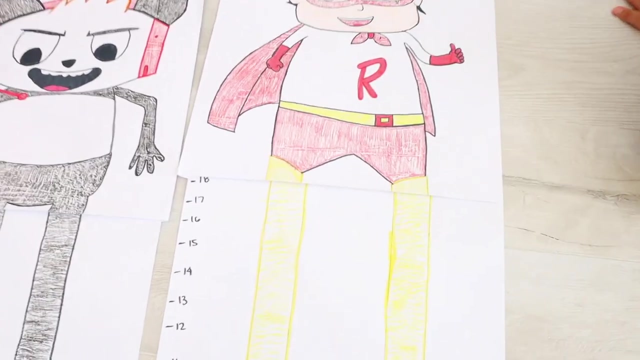 Both of them are teenagers. Yeah, Okay, but now I'm going to be older than Combo. Well, we'll see Boom Again four, But he's just going up by four every time. Ooh, 18.. Are you ready to go up in college? 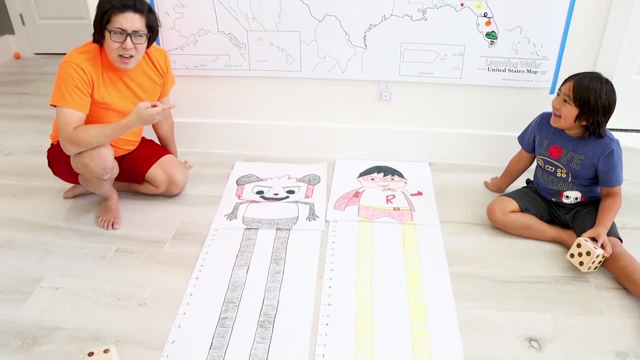 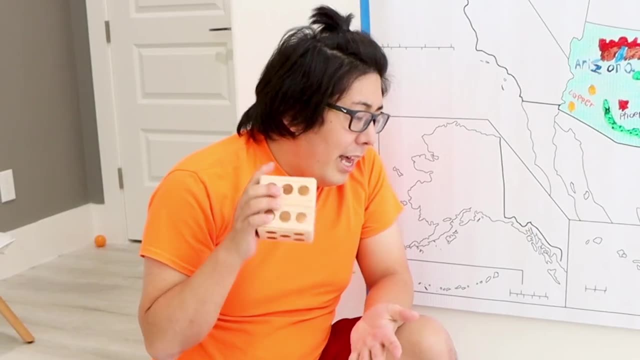 Wait, if that's, Did you take SAT ACT? Yeah, Which one Combo Daddy? if you get a four, five or six, you win. Right When I hit 20, that's when I win. All right, here we go. 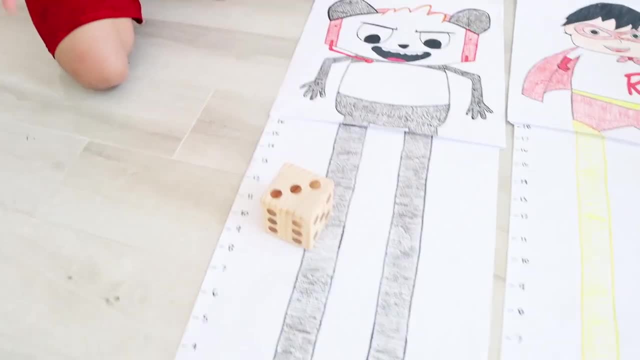 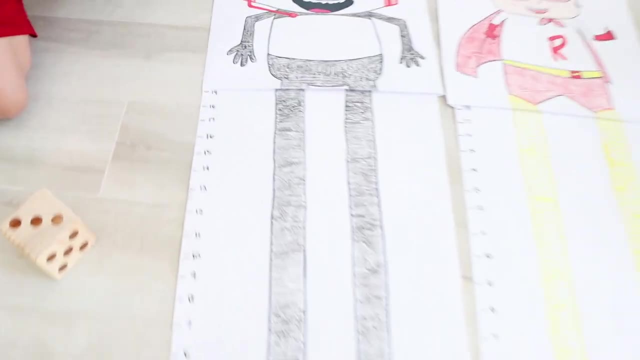 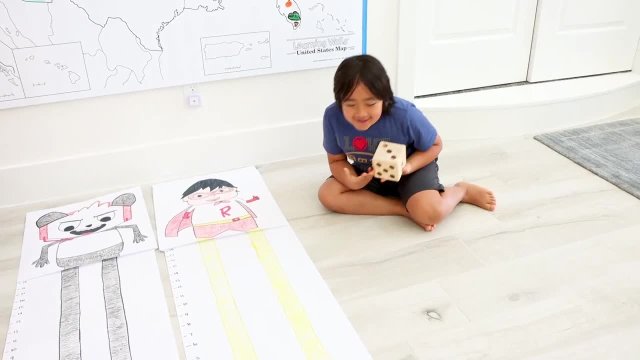 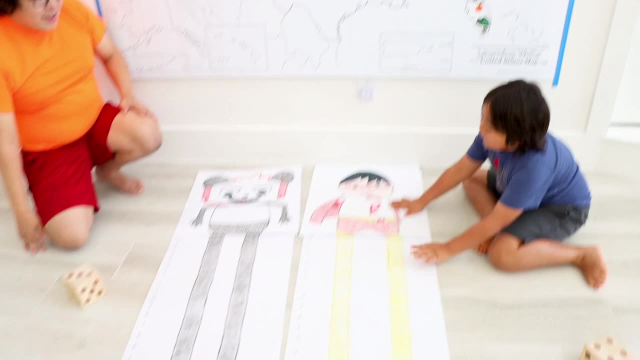 Can he do this? Probably? Okay, three, two, one, One, Yay, Ah, he got it All right. roll, Roll forward. Oh gosh, Oh, what happened to his leg? Oh, no, no, no. 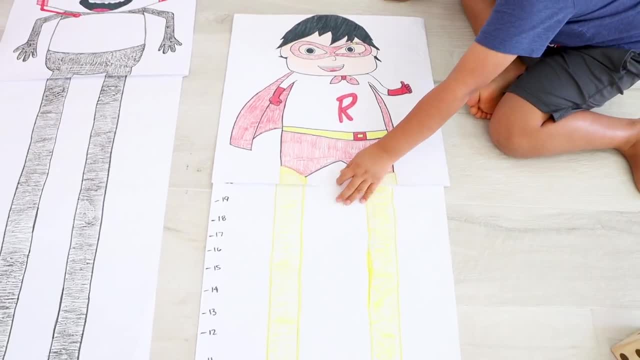 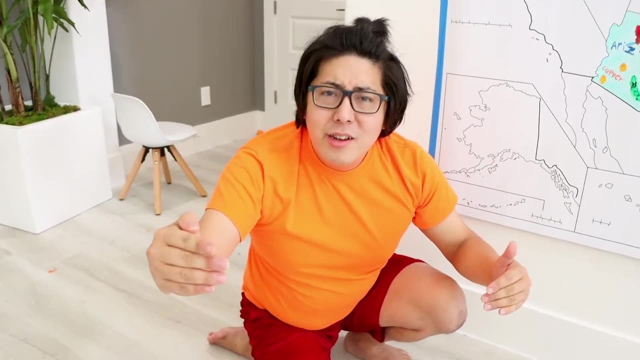 Hit it back, He dislocated his leg. There you go. Yay, I won, I'm the first to get to 20.. It's okay, We're gonna do one more round. Okay, so this time, instead of growing legs, we're gonna grow arms. 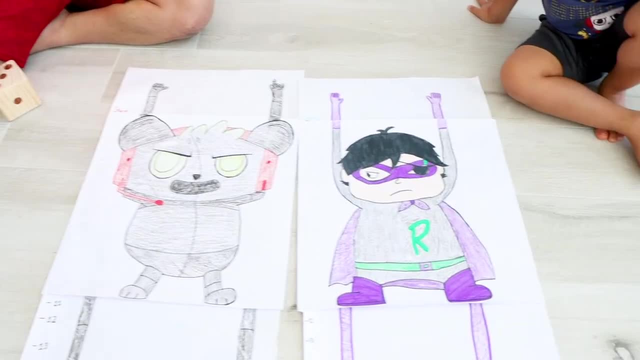 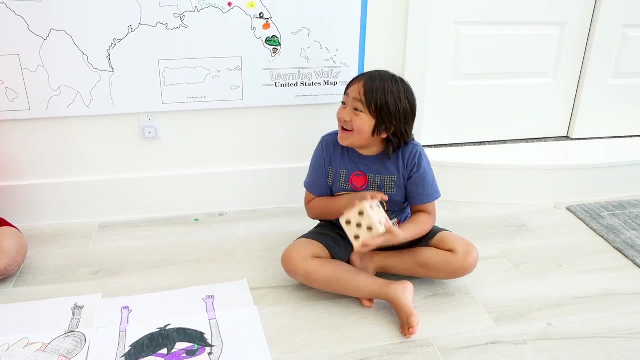 So it's gonna be between Robocombo versus Dark Titan. Who's gonna have the longest arms? I don't know. Well, I'm gonna go first. To be honest, though, guys, I think they need the longest leg. Look at their leg. 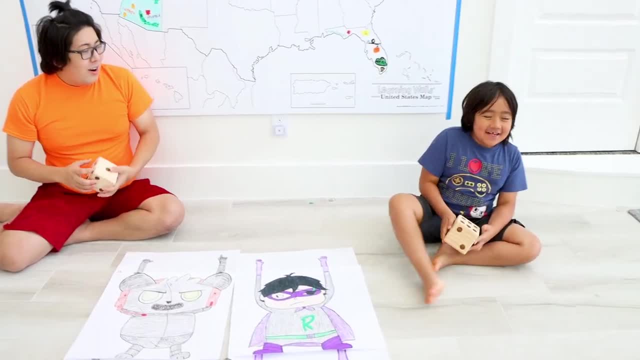 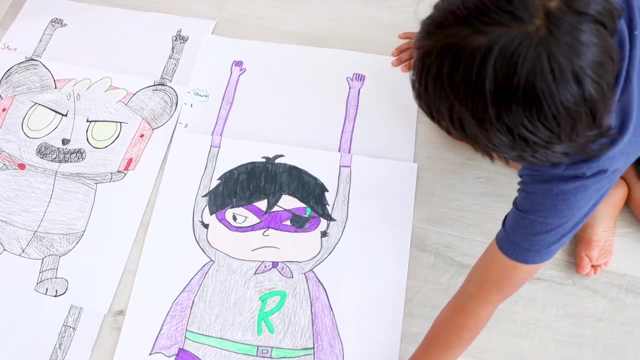 Very short, Yeah, But it's okay, We're gonna work on the arms first. Yeah, Okay, let's do it Two. Aw, Starting out slow, Smart. That's why he's upset. Look, Look at his angry. 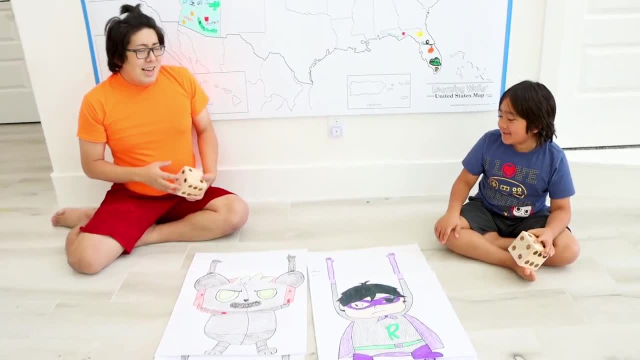 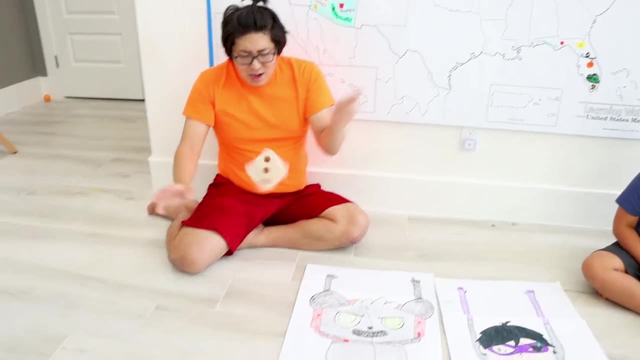 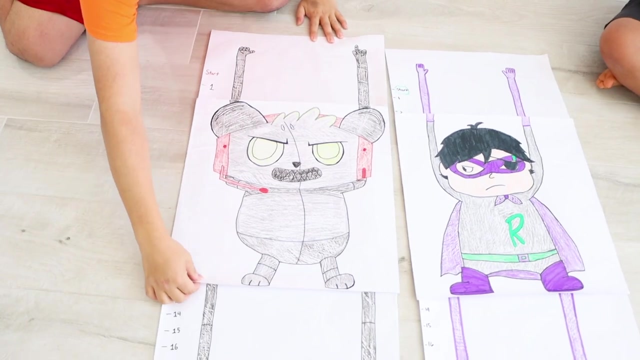 Mm, Mm, Those are already very long arms. This Robocombo looks happy. He's smiling, I think. Why just his face? I don't know. All right, here we go. Six for the winner. Boom, boom, boom boom. 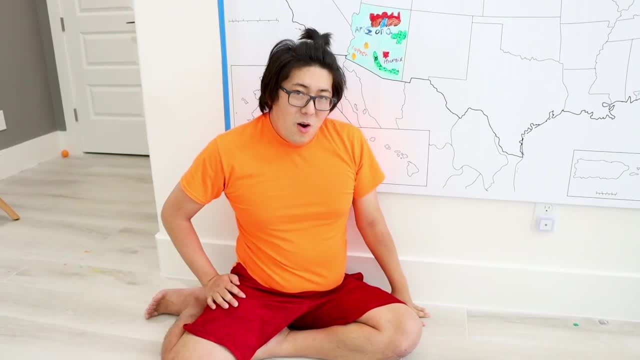 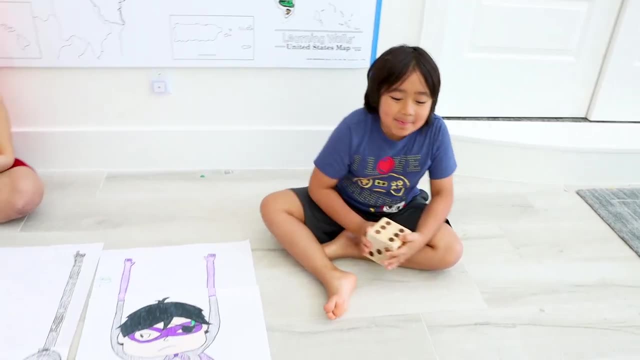 You always get six in the beginning. Oh, whoa, I mean, he's a robot, so all he needs to do is extend his arm, right, Yeah, Okay, I'm going to speed five. Good job, So now I'm one better. 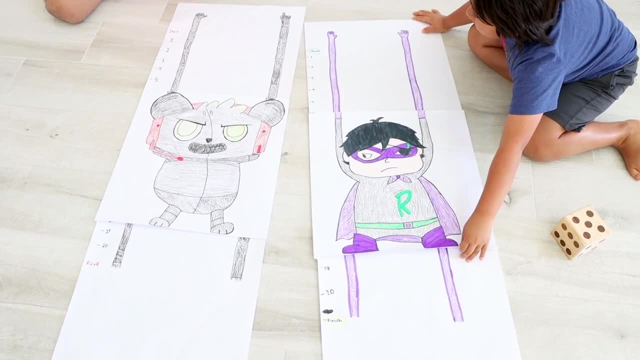 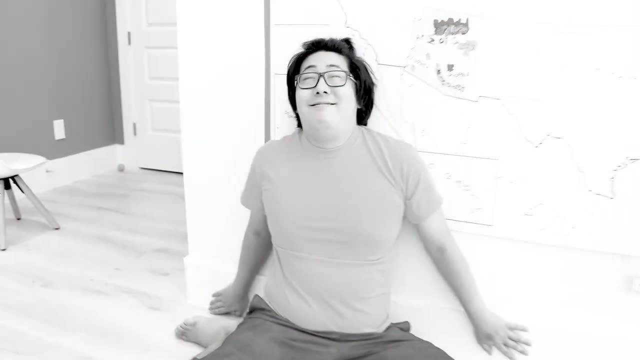 That's true, You're ahead of me by one. One more Wait, or oh, yeah, You're at seven. Yeah, Good job, Ready. Oh, Good job, Ha-ha, Ha-ha, Ha-ha. 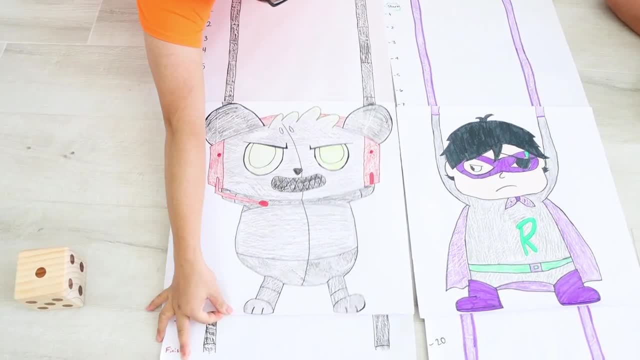 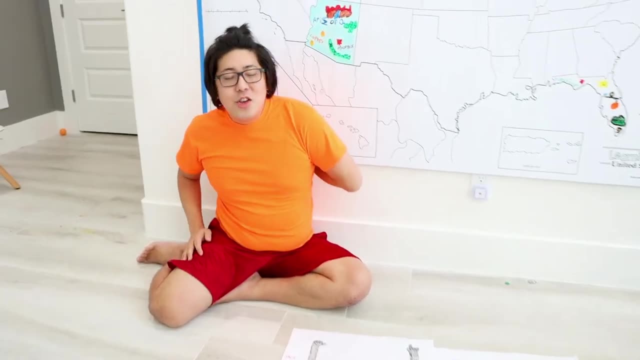 Ha-ha One. It's okay, We can retie. We can retie He had an error on making him his arms longer. Oh No, All right, Your turn, Ryan, Just go, Just go Okay. 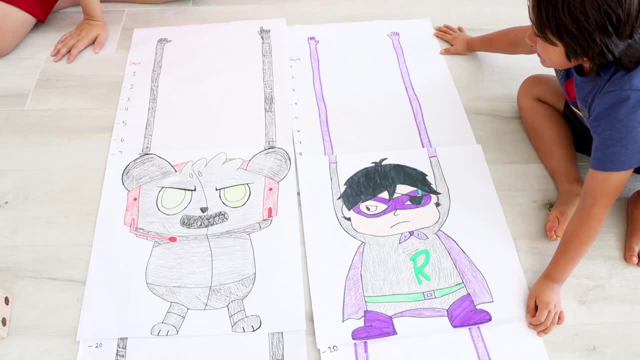 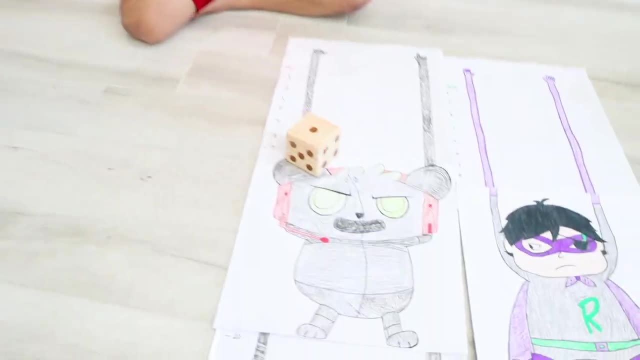 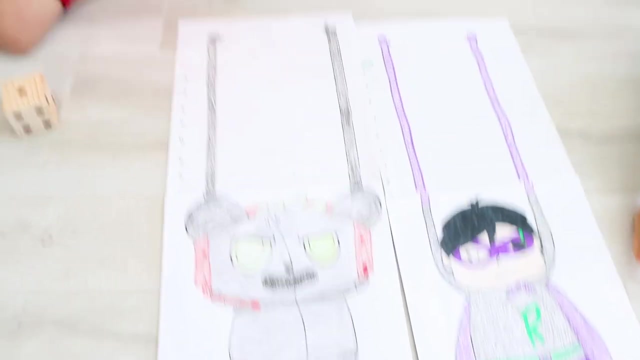 No, I got two. You're going very slow this time. All right, This is going to be the Evo with the longest arm. It's going to be a robot combo. No, He had another error Again, I can't even tell the difference. 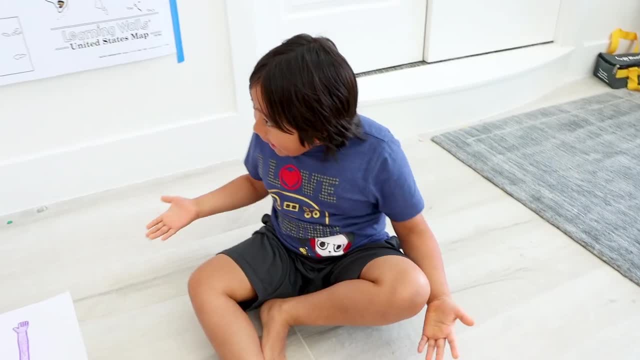 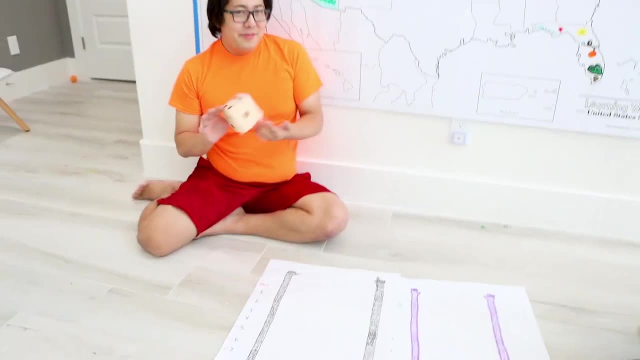 Very subtle Boom One. You get one, I get two. This is very anticlimactic. Ha-ha, Ha-ha, Ha-ha. This is what people buy a ticket for- Ha-ha, All right, All right. 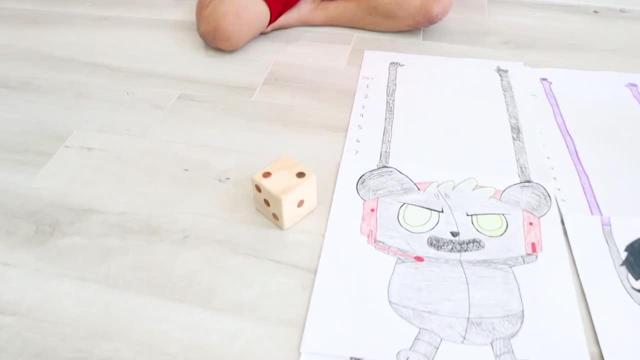 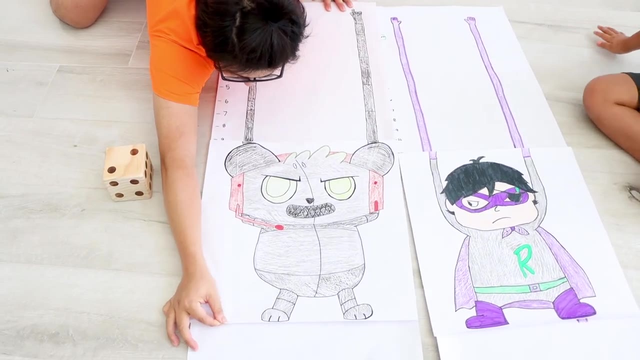 Play, play, play. Give me, Give me good luck. Ha-ha, Ah, That's slightly better. Ha-ha, He got slightly better. Well, maybe I'll get three, One, Two, Two. Okay, I'm halfway now. 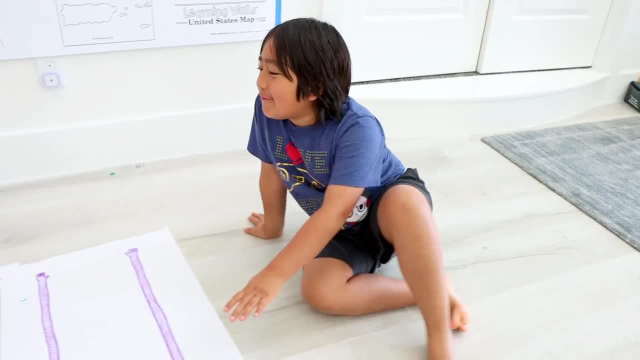 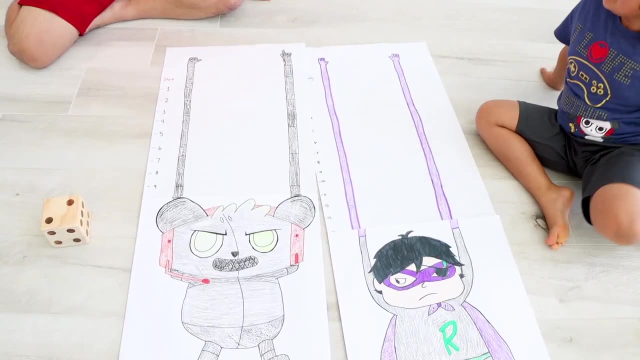 Okay, Let's see what I got. I got three. I always get one more than you. Yeah, That's okay. All right, Keep going. Uh-huh, I got 14.. Yeah, Look at the arms. It's so long. 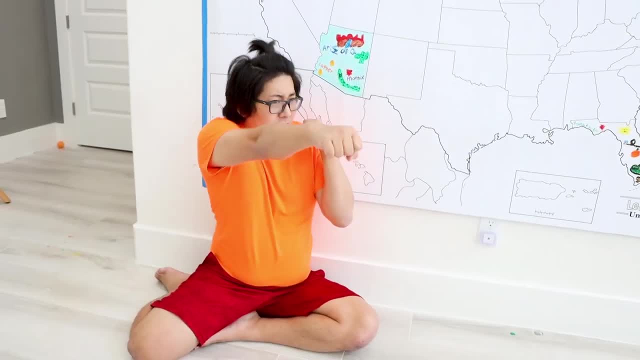 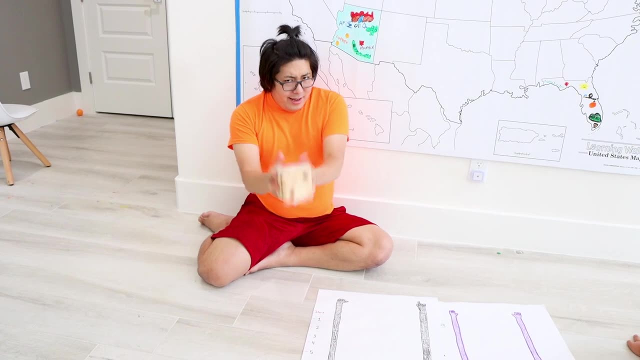 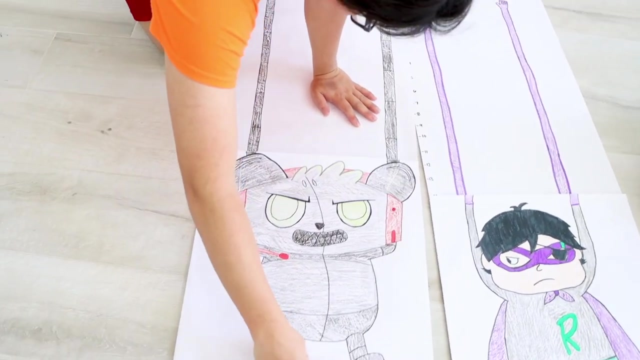 He's 14 arm old. If they punch they can just go all the way over there. Yeah, Ah, Poof, Ha-ha, Ready, Whoa. Wait, Does it count? Sure, Okay, One, two, three. 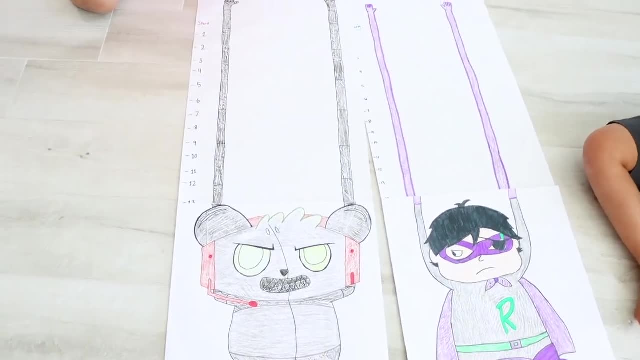 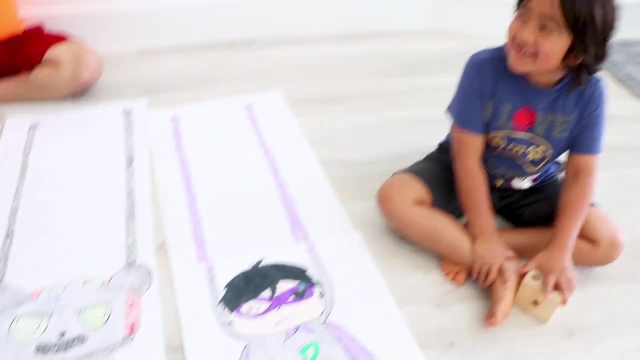 13.. Oh, that's a bad luck, Ha-ha. Right now, Roblox combo is 13 and Dark Titan is 14. We're in our teenage years. Ooh, I do not like that. It's a lot of work for parents, teenagers. 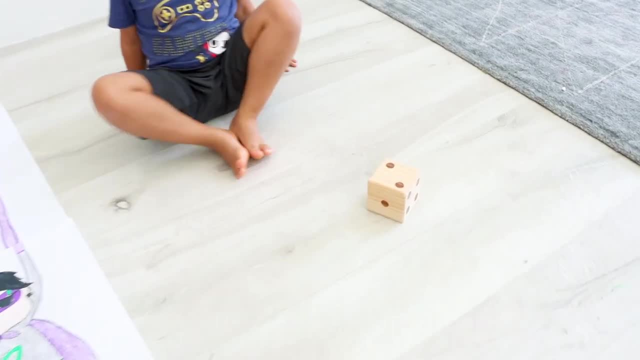 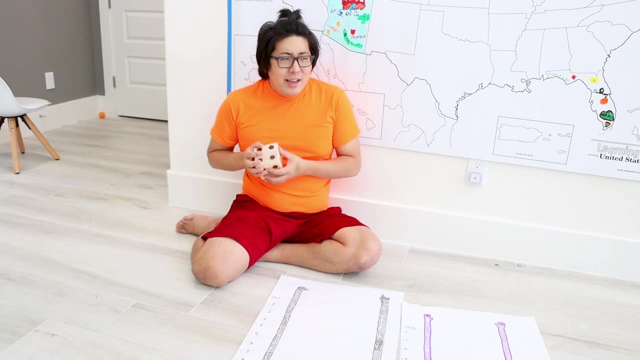 Okay, Three, two, one, Two. All right, I still have a chance to catch up. No, you don't. You don't have a chance to catch up. I catch up, I love to catch up, All right. 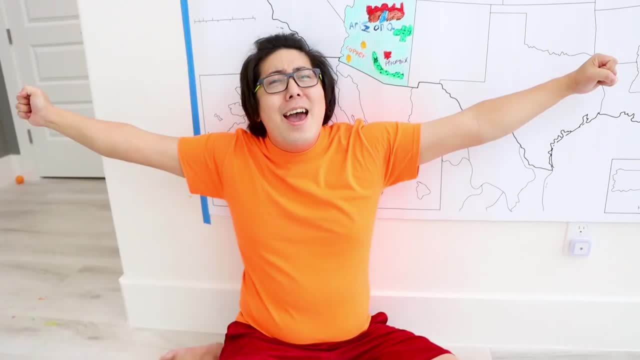 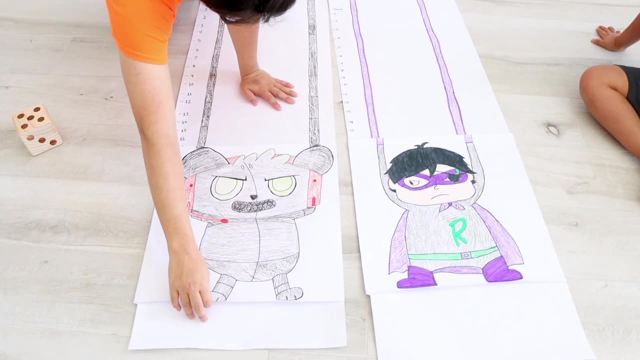 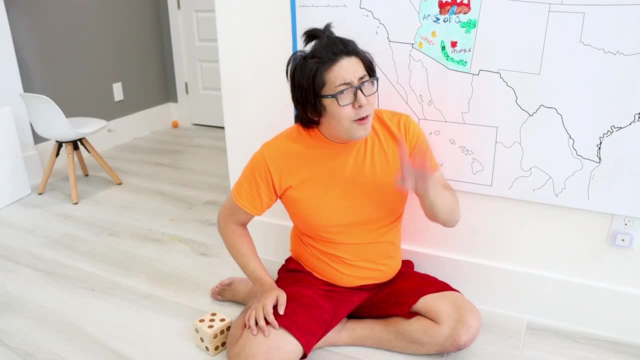 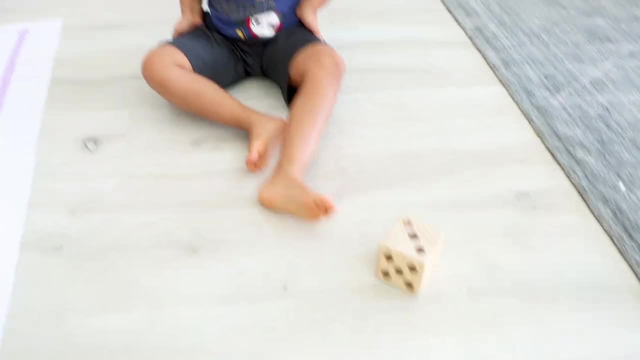 18.. If Ryan gets four or more, he wins this round. Let's see if he can do it. Three, two, one, Ah, All right, Go up three, It's okay, I still might not win, okay. 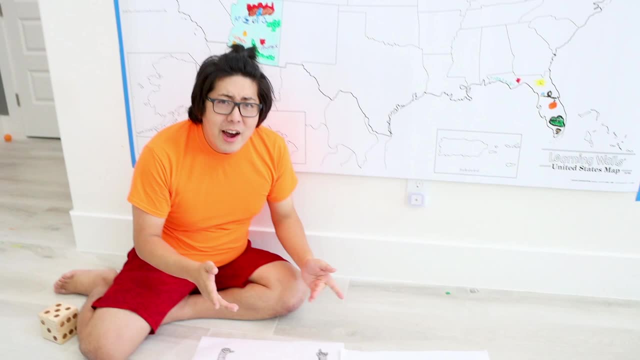 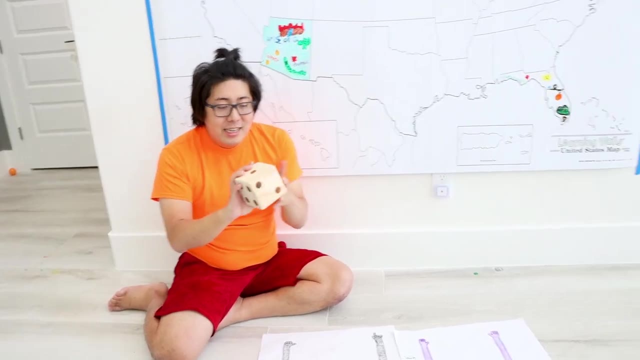 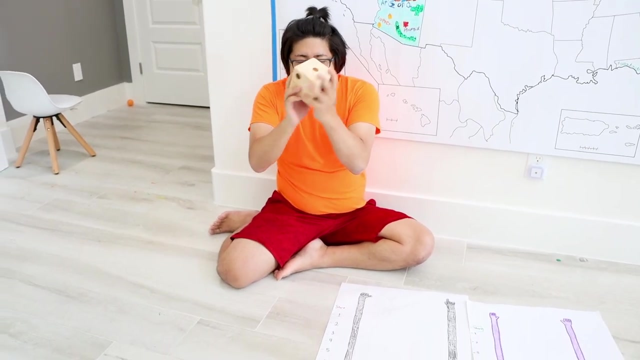 If you get one. So Ryan's at 19 right now and I'm on 18.. So this round, if I roll one, any other numbers I'll win. Here I go, get one, get one, get one. 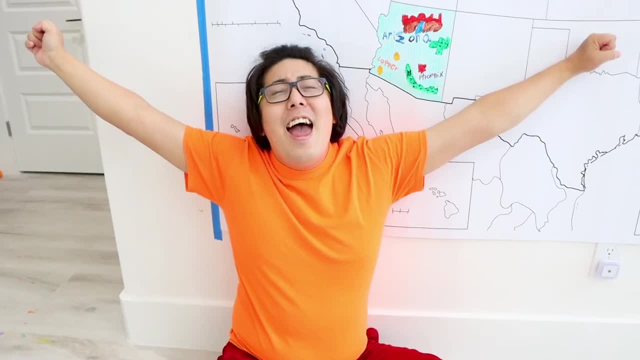 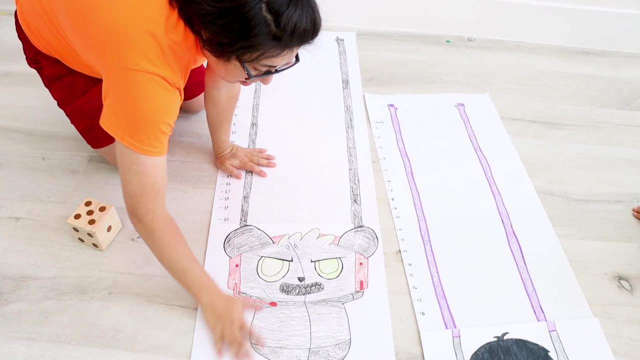 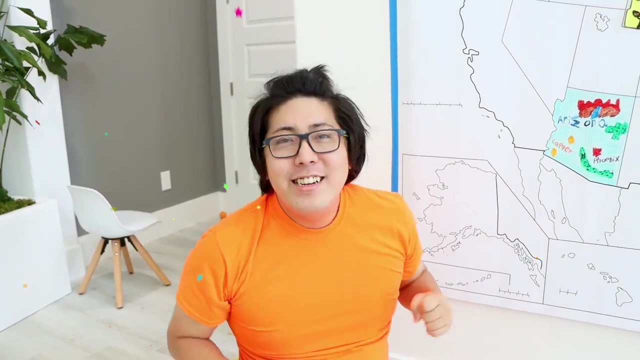 Come on. Yay, He goes in beyond. He goes 23,. so Get right here. Yay, So it's round two. I won. Now we're going to show you how to make your own DIY game. Roll the clip. 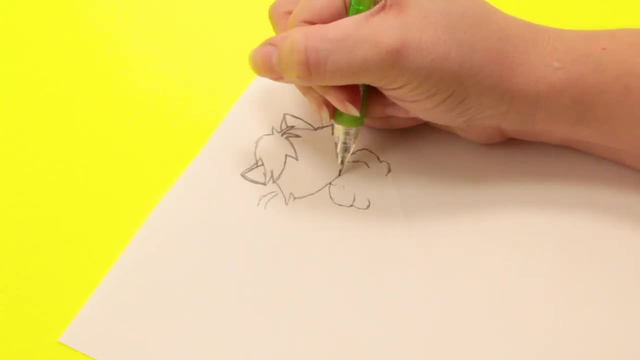 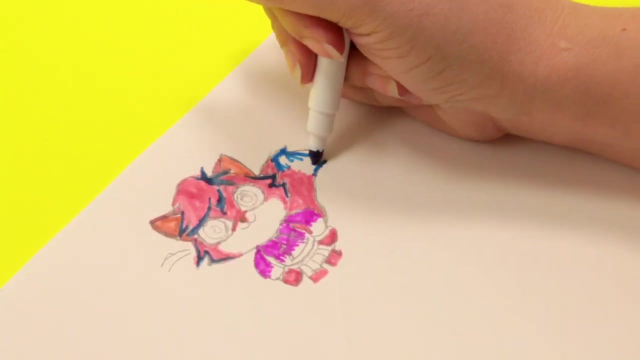 I'm going to start by drawing my favorite character. I'm using pencil so I can get all the little details Next up. add in color. Now. Alpha has lots of pretty pinks and blues and all sorts of colors that make her Alpha awesome. 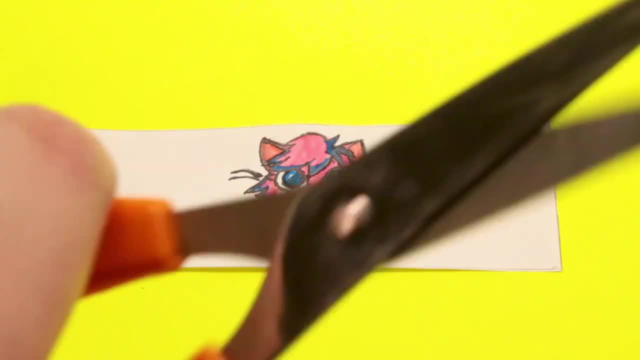 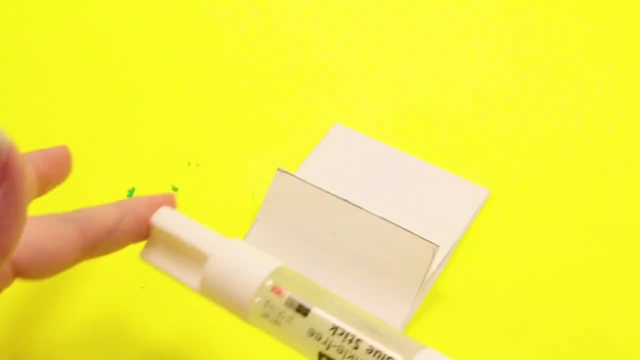 There. Now I'm going to cut her out into a rectangle and make the outer sleeve. I need to fold it into thirds, but make sure I leave a tab that can be glued together, Something like Like this: Next up, making the counter board: 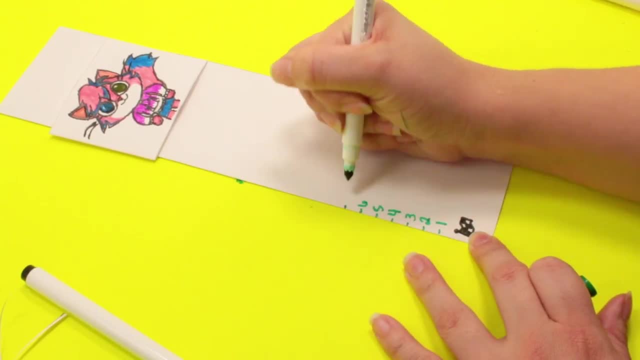 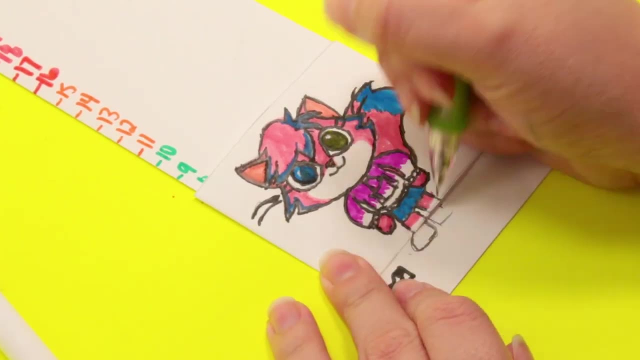 I've folded a piece of paper in half and glued it together. Now I count all the way up to 20.. Perfect, Now we need to add the feet. I'm going to sketch out the feet and then stretch all the way up and connect the legs with a ruler. 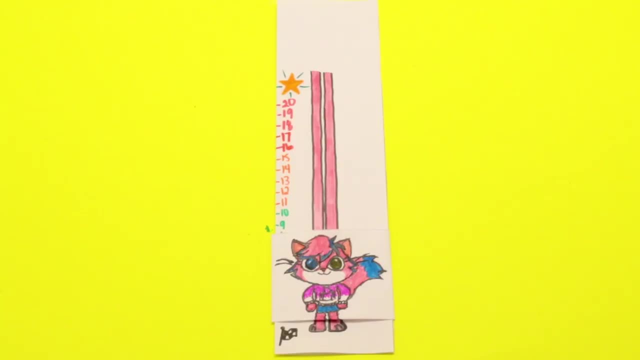 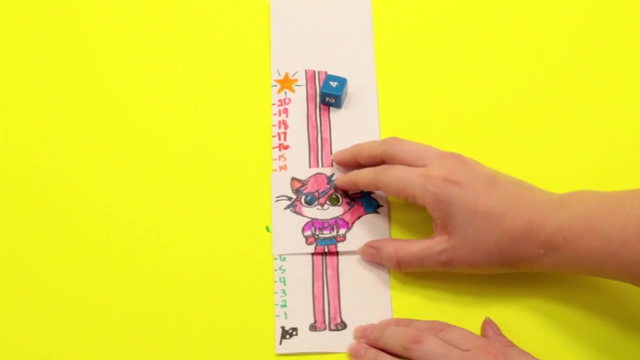 Last step: coloring the legs. And. And you are ready to go, Let's test it out: Three, One, two, three, Let's try again. Four, five, six, seven. Once you get all the way to 20, you win. 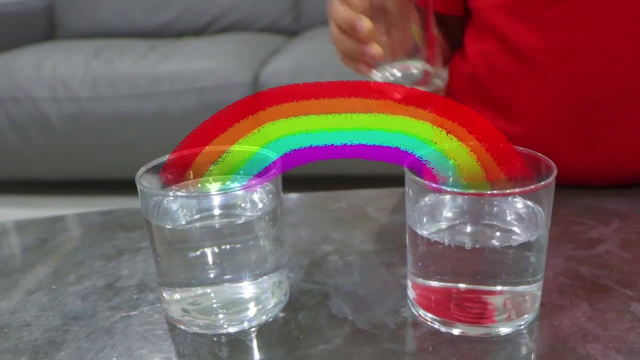 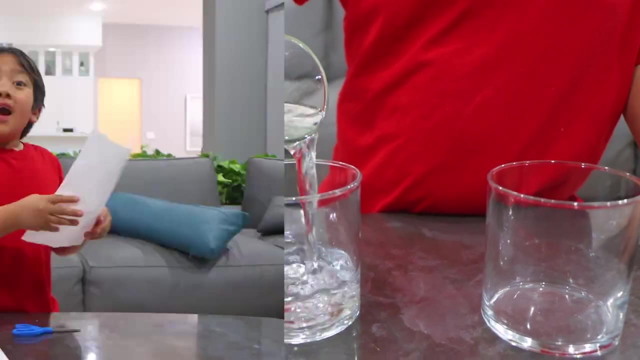 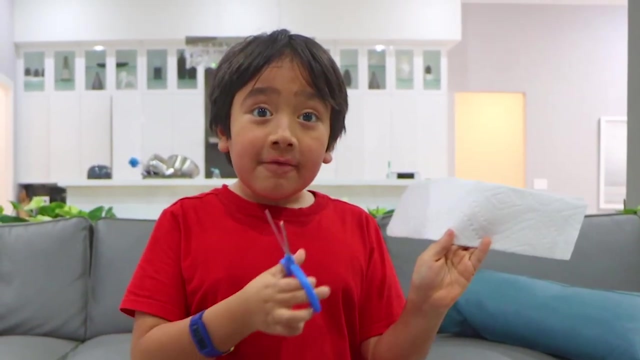 Hey guys, today we're going to grow our own rainbow. All you need is a paper towel, scissors, markers and cups with water. First, using your paper towel, you're going to fold it in half, Then we're going to cut it one-fourth. 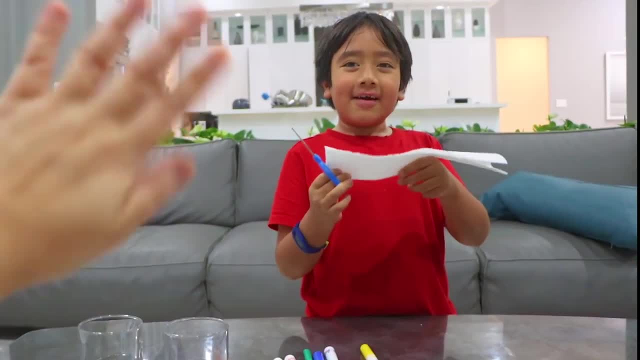 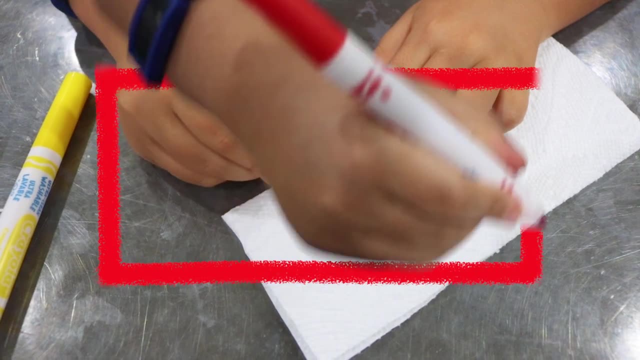 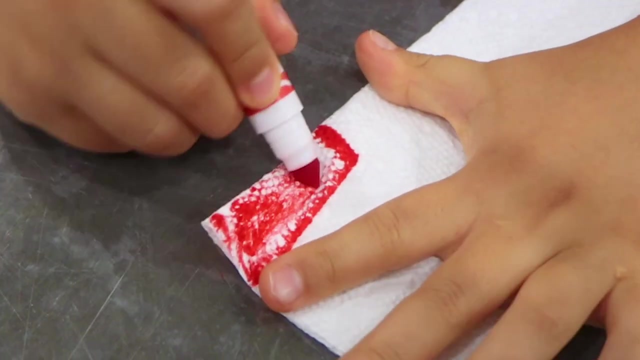 Don't forget to ask a grown-up for help, And I have mommy here. Hi, Hi, Thank you. So first, with any marker you want, make a rectangle like this. Now let's color it in. The next color in the rainbow is orange. 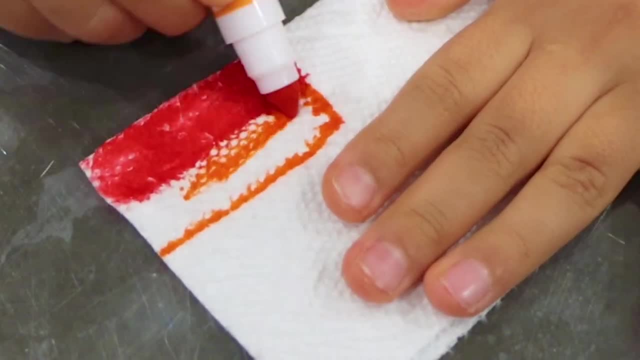 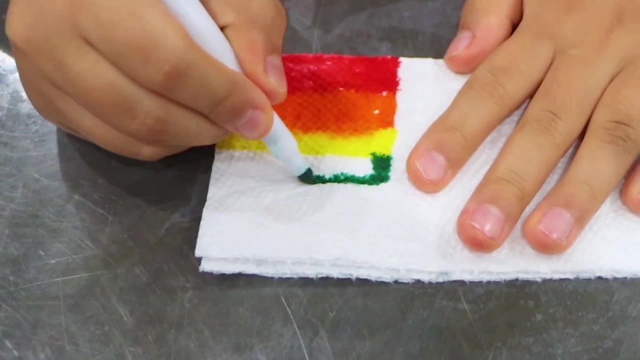 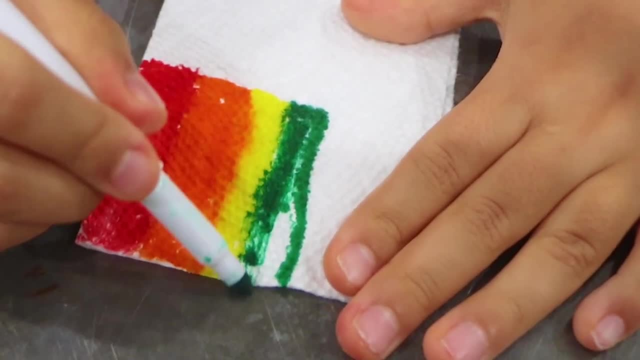 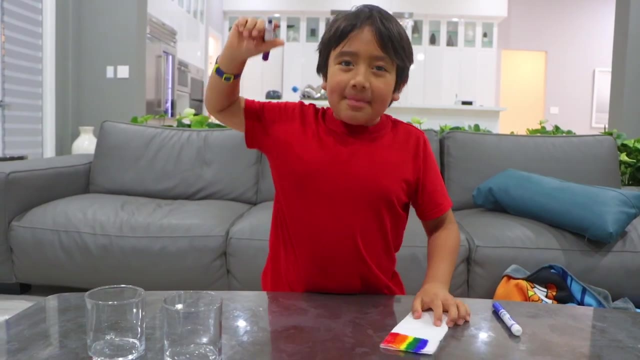 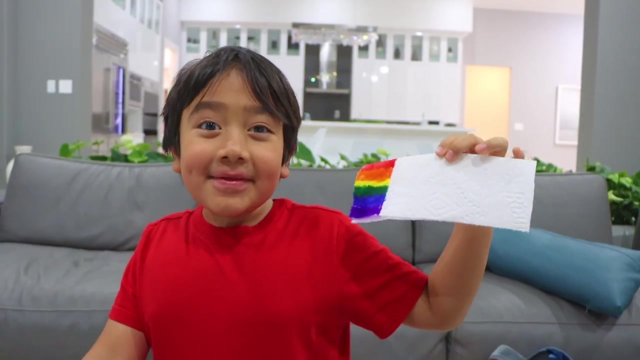 Let's fill this in. Next is green. Fill it in Green. Next up is blue. We're going to finish it off with my favorite color, purple. Now do the same thing to the other side. Like this, See, like so. 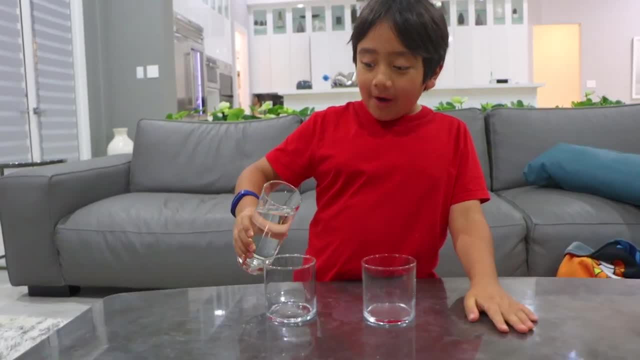 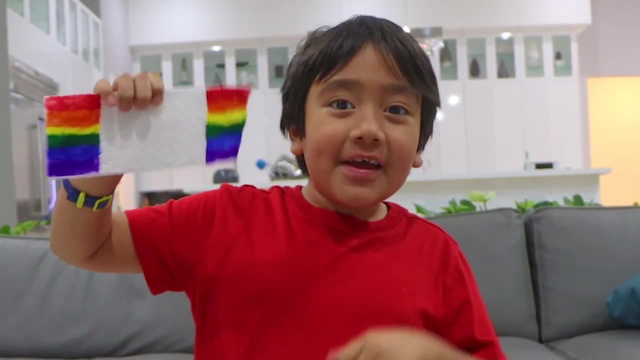 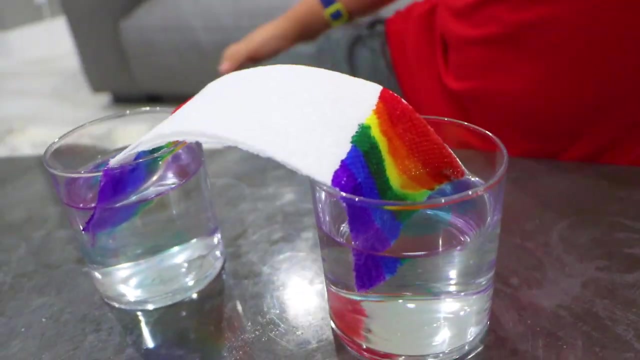 Next, fill up your two thingies of water. There you go, There you go. and the second one. Now take your rainbow paper that you drew and put half of both of the sides in the water. Now we wait. Watch the rainbow form. 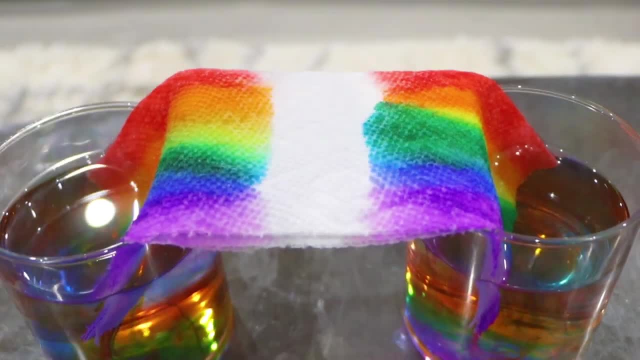 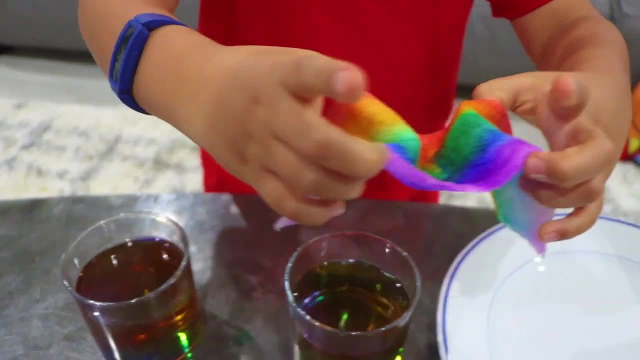 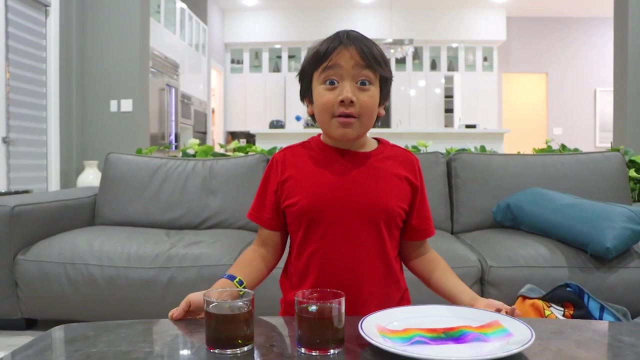 Look, it's already forming a little bit. Whoa, guys, did you see? We made our own rainbow? Whoa, Put it right here. This is so cool. Did you see the marker die? move up the paper towel and touch each other. 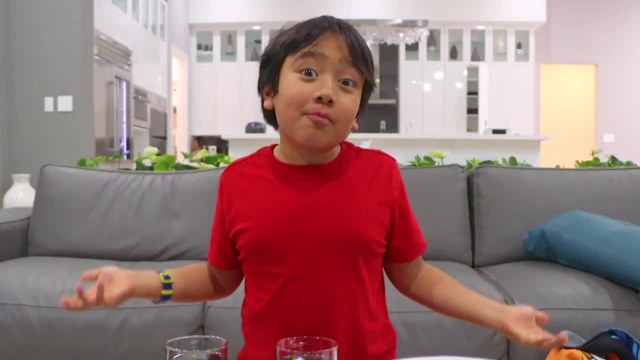 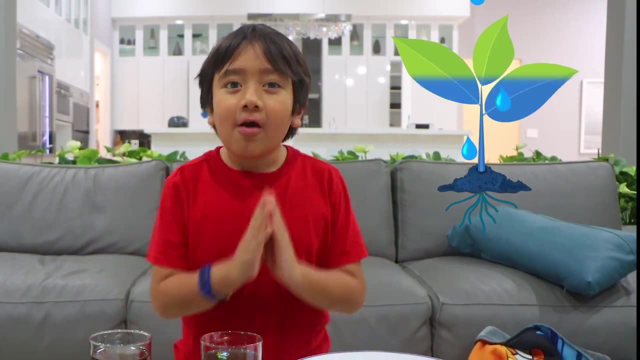 Cause that's called capillary action. Did you know regular plants also use capillary action? Cause they bring the water from the roots and make it go all to the other parts of the plant. I hope you guys had fun making our own rainbow together. 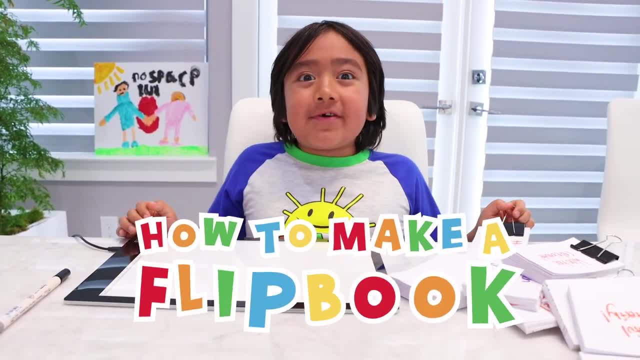 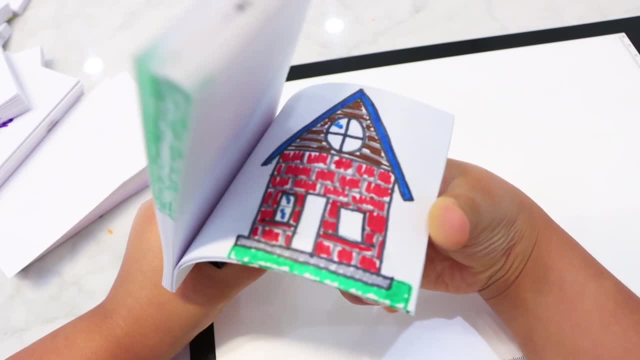 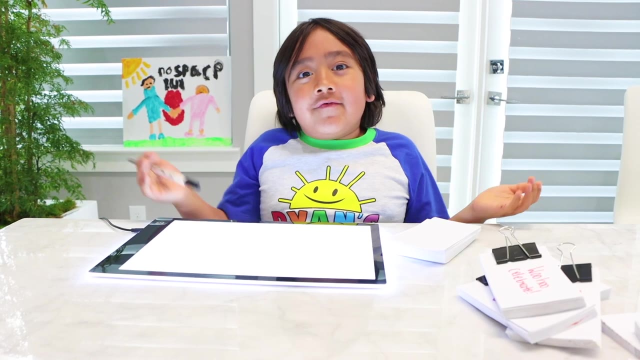 Hi guys, today we're gonna be learning how to make a flip book like this, And this one is called Home, Sweet Home. In this one, a house is built, So all you need are some flashcards, a light box and, if you don't have a light box, 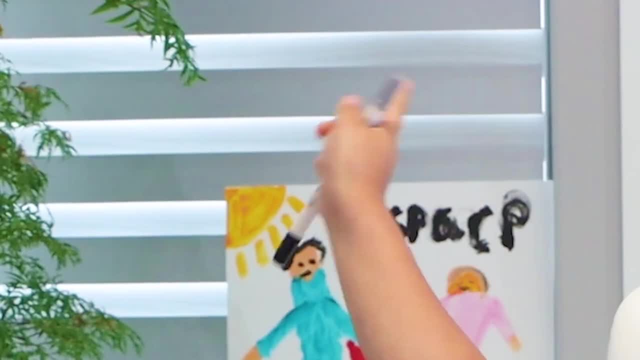 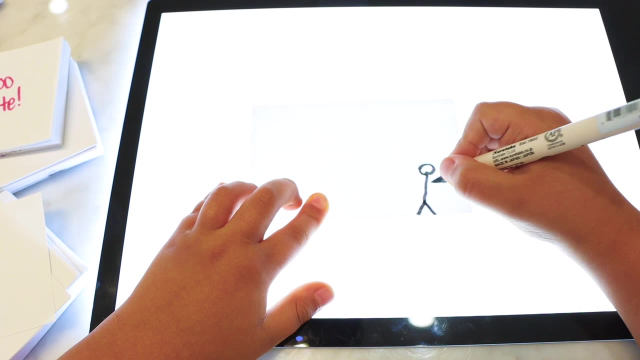 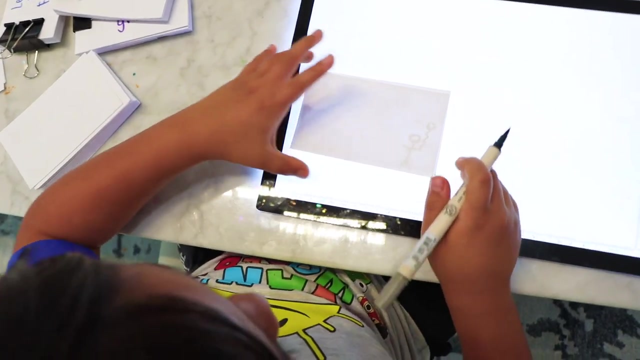 or something else that makes light, then maybe you can use the window and you can use marker. First I'm gonna draw a stick figure man on the side of a flashcard right here And maybe he could be holding a balloon. Next Put another flash card on top of it. 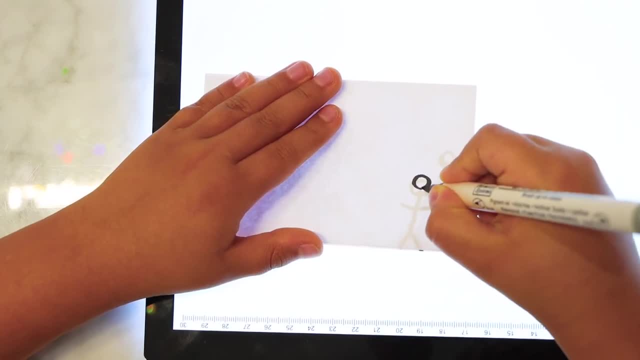 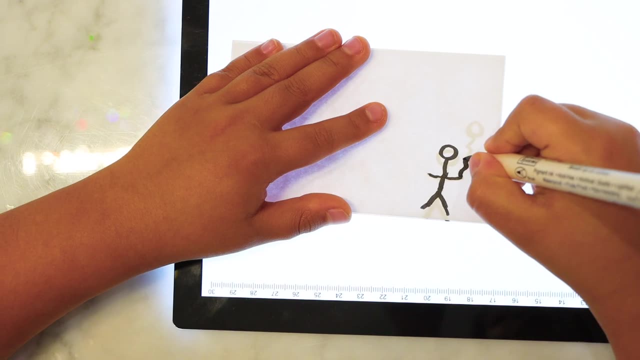 And make sure everything is lining up And then draw whatever your thing is how it's gonna look like on the next page. Like maybe mine is gonna go a little higher, Then you're gonna keep doing it, So put the bottom sheet over here. 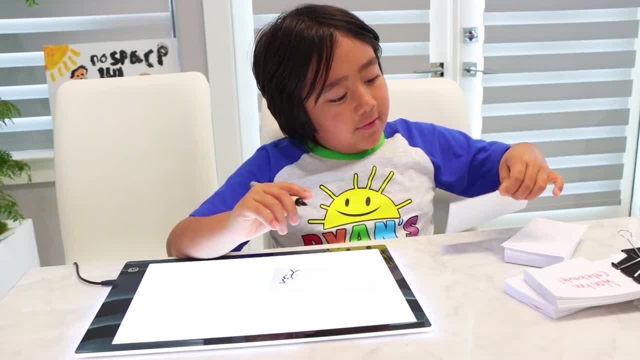 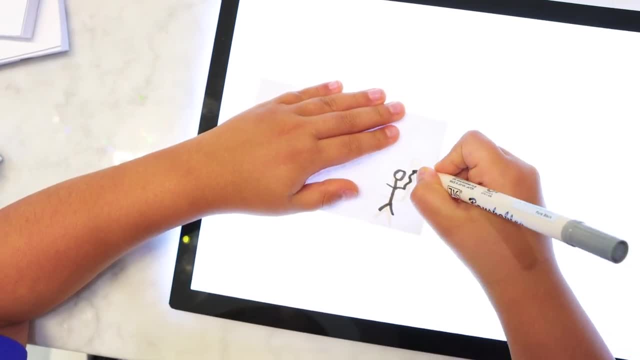 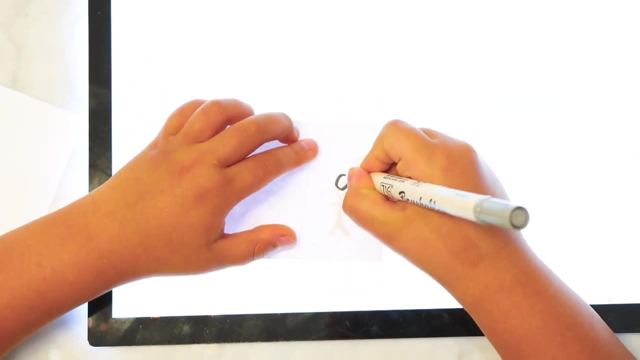 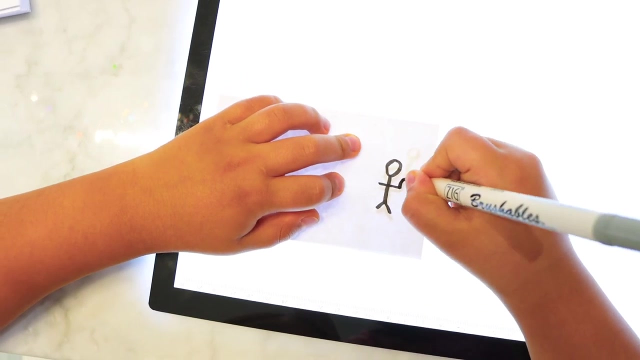 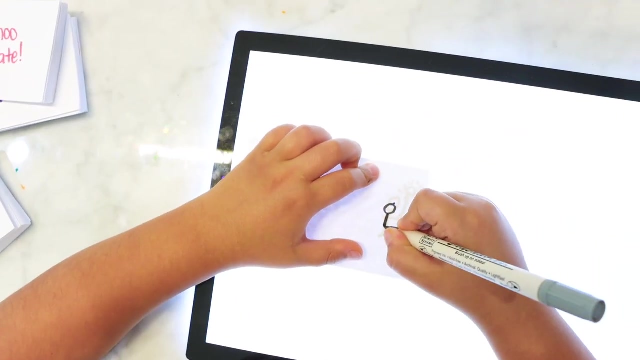 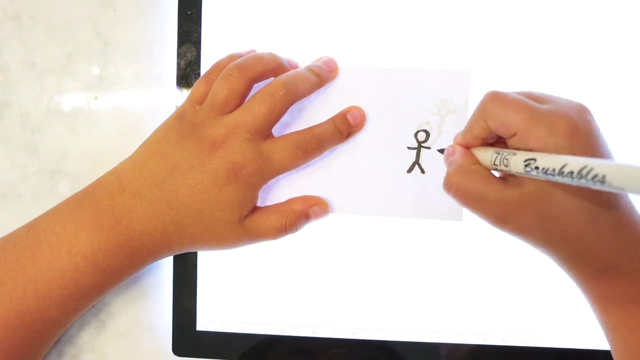 And draw him like this with the legs and the balloon. Okay, I'm gonna keep doing this over and over again until the stick man and the balloon gets higher and higher. Uh-oh, the balloon just popped. Ah, I'm drawing him falling. 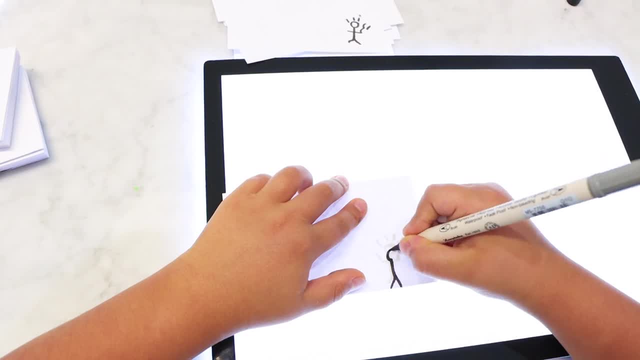 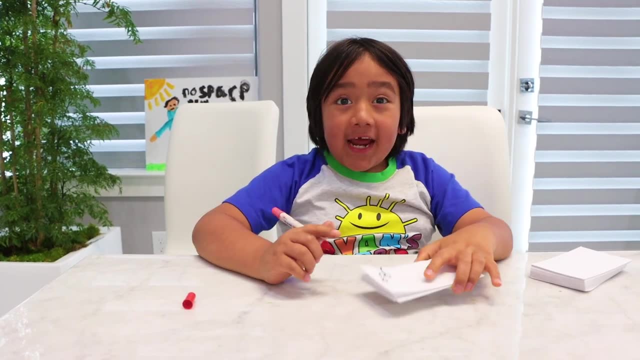 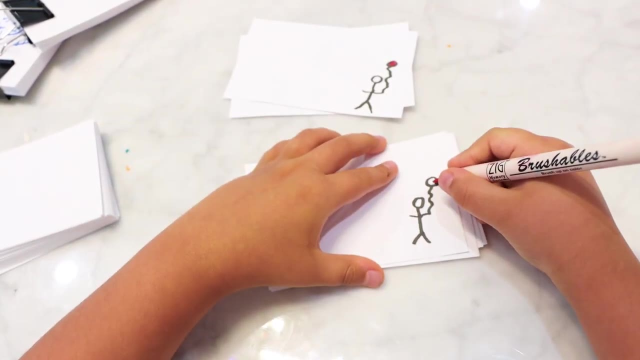 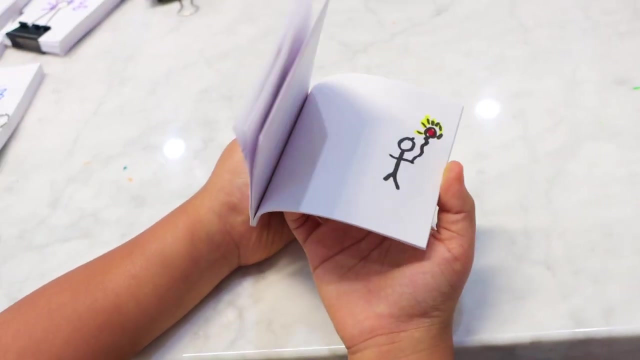 Once you've finished your drawing, you've gotta put it all together, And now, next, I'm gonna color all my balloons. Okay, guys, I'm all done. Let's see it in action. Okay, so that was my super simple. 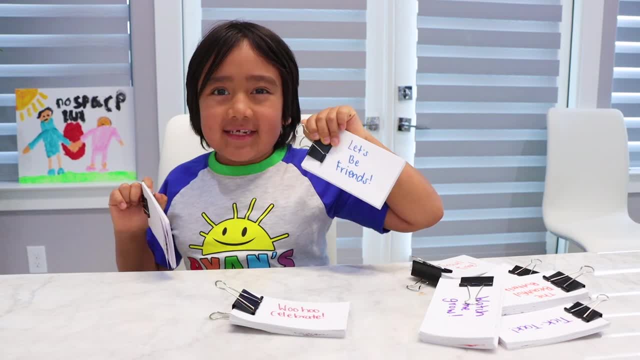 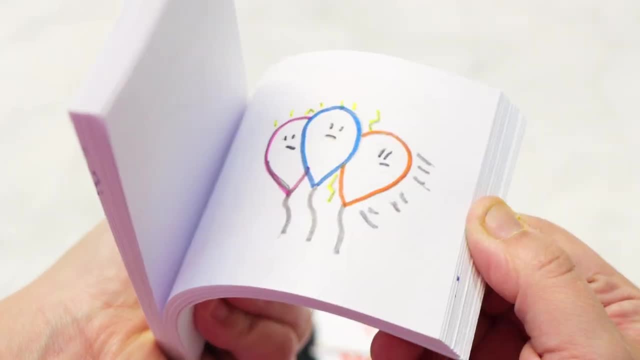 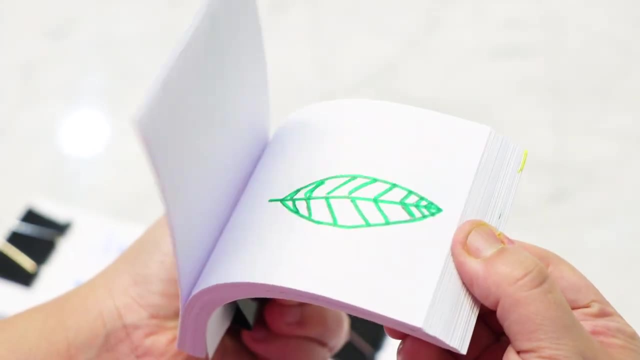 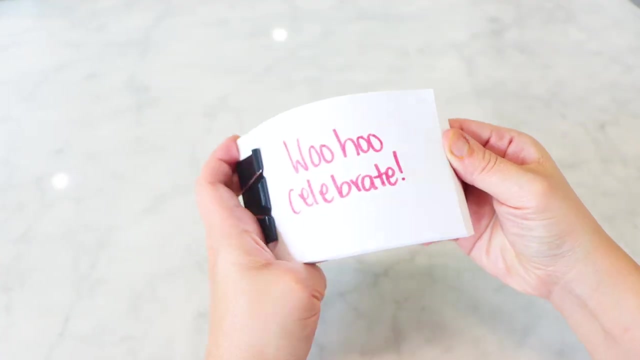 balloon drawing. And here's my flip book. And here's some other flip books that you can see. This one is called Let's Be Friends. This one is called The Beautiful Butterfly. This one is called Woo Hoo Celebrate. This one is called Travel Time. 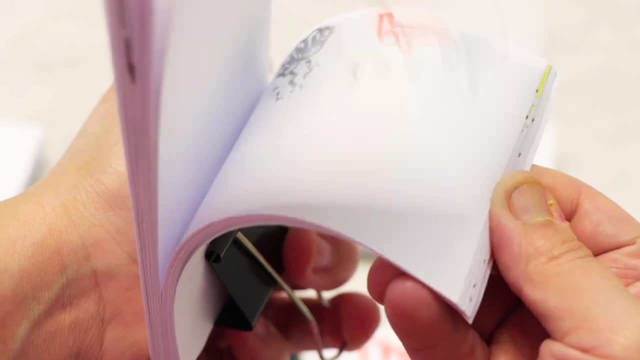 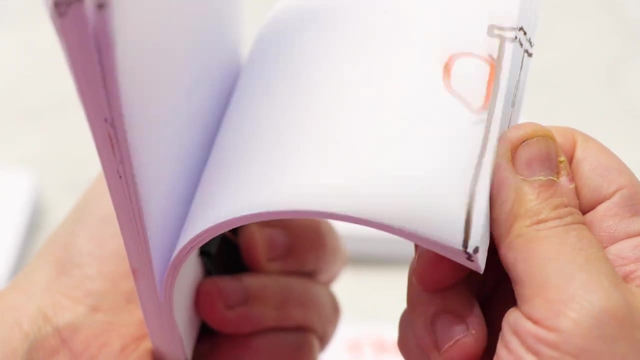 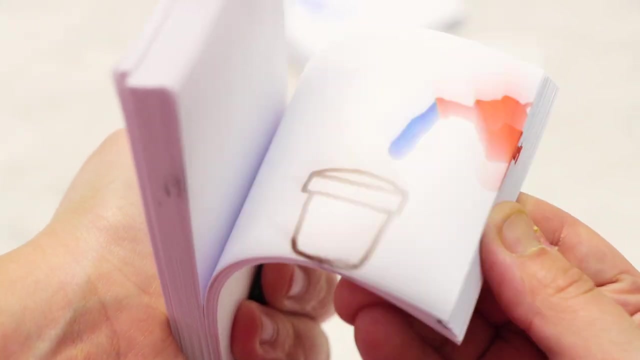 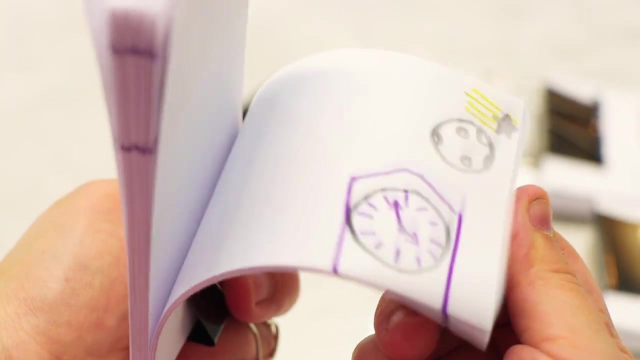 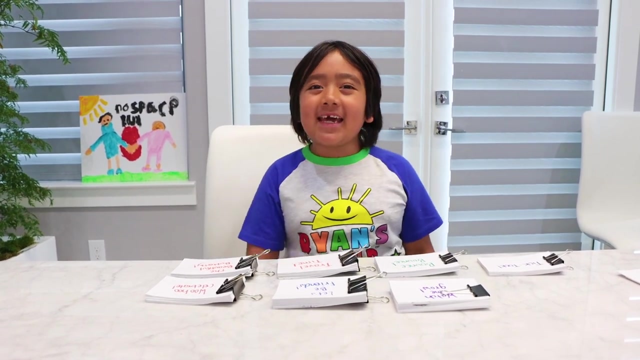 This one is called Bounce Bounce. This one is called Watch Me Grow. This one is called Tick Tock. Thank you for watching our video. Hope you enjoyed learning how to make a simple, easy flip book with Ryan. Hi guys. 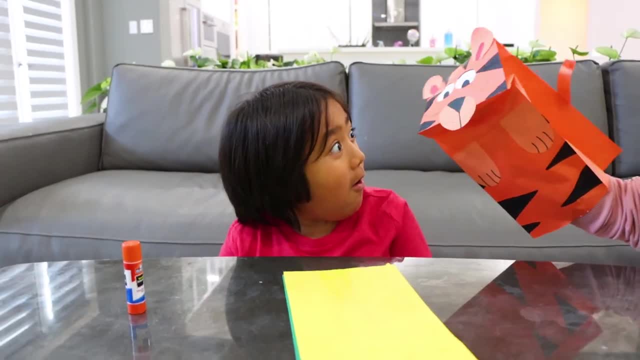 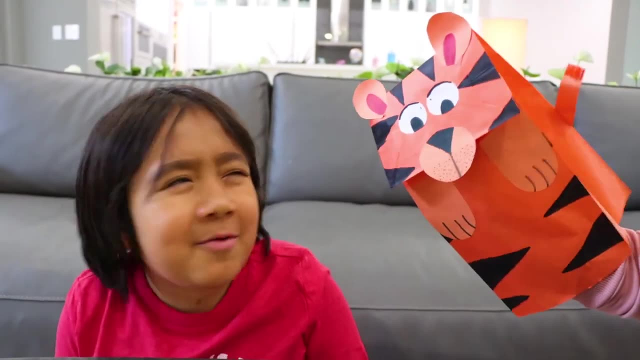 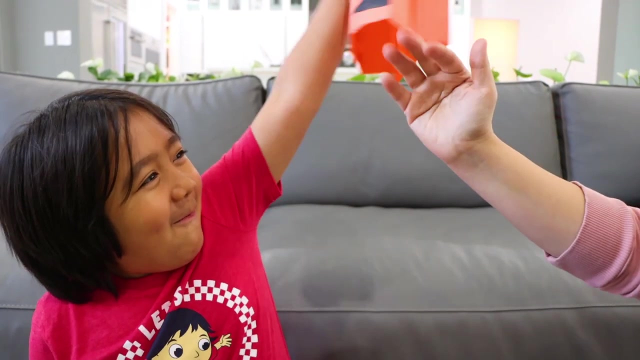 Welcome to Ryan's World Today. who are you? I'm Tootoo the Tigeroo. I don't think you are. You kind of sound like Mommy. No, I don't. I'm a real tiger. Grr, grr, I mean grr, grr, grr. 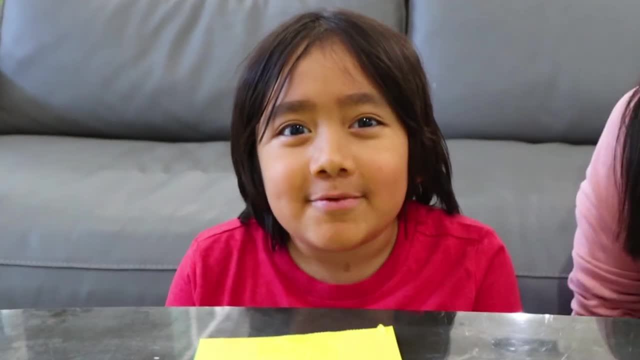 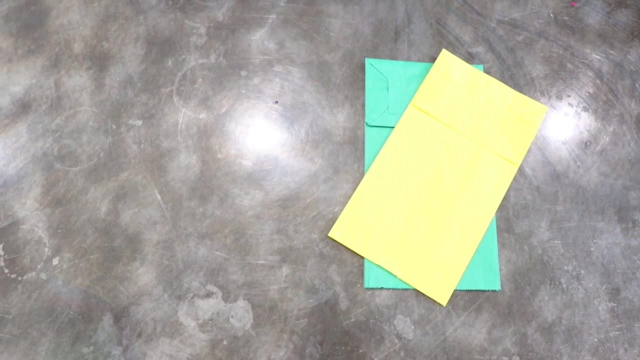 Okay, I'm Mommy Hi. So, as I was saying, we're gonna make paper bags And we're gonna cut out the parts that we need to make a giraffe into animals. Let's get started. So all you need is paper bags. 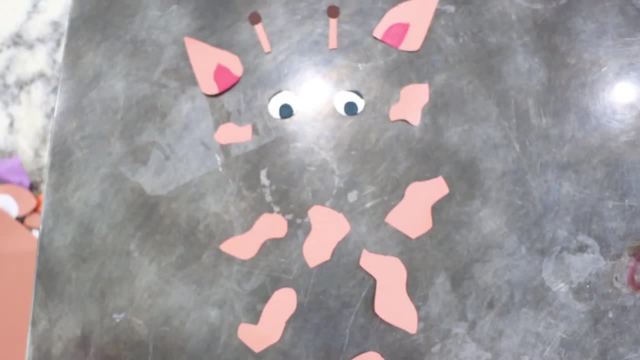 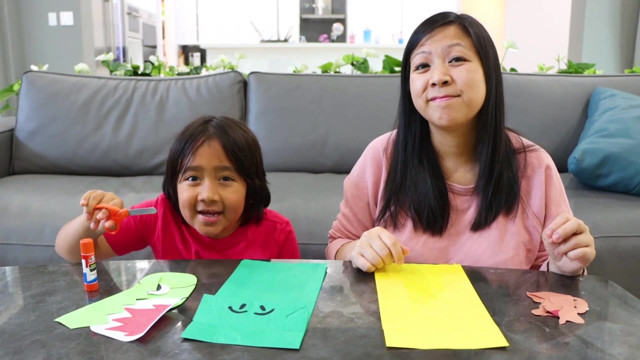 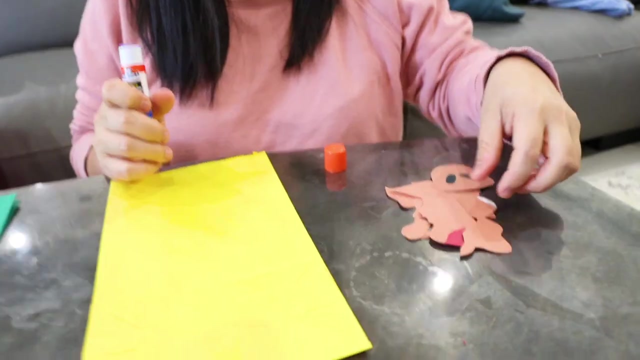 construction paper. glue and scissors. Cut out the parts of construction paper like this: Okay, so I cut out all the parts I need. Now I'm gonna make an alligator And I'm gonna make a giraffe, Okay, so all we need to do left is glue it. 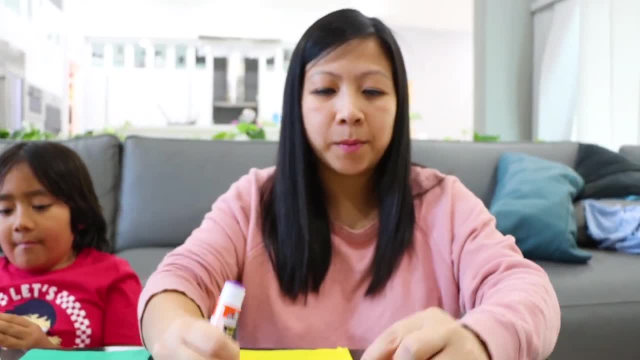 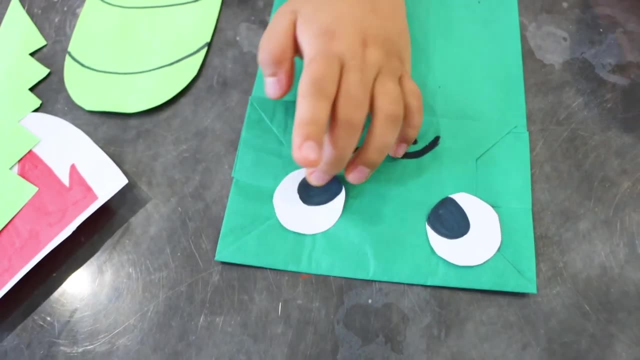 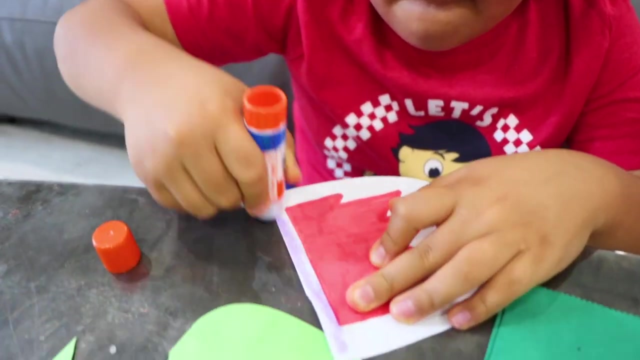 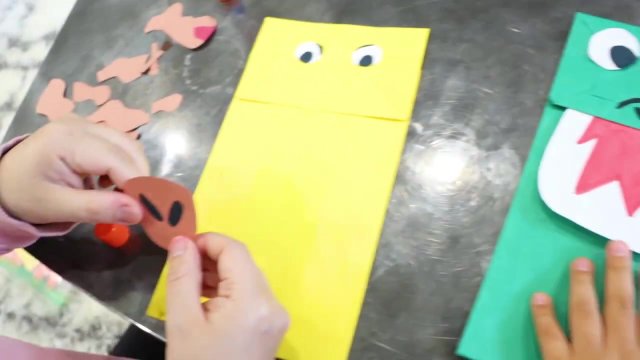 Okay. so first, the gap is the eyes. I'm gonna glue the eyes right here. Okay, the eyes are done, Oh there. Then I put the mouth, Boom the mouth. I have a giraffe nose right there. 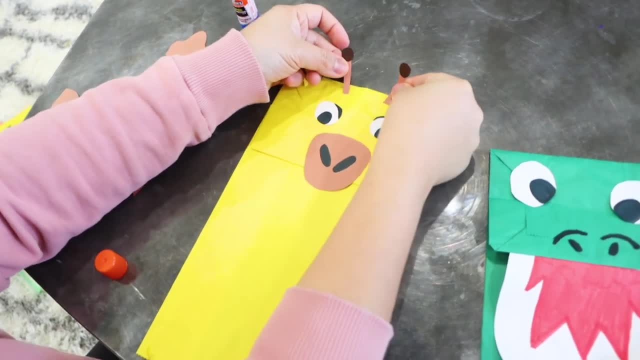 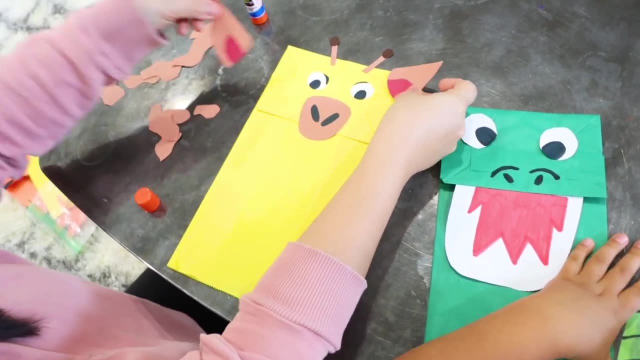 so you can smell. That's important. And then giraffe: It has little horn that looks like antennas right there, so I'm going to glue that there, And then I'm also going to glue its ears like this. Does it look like a giraffe yet? 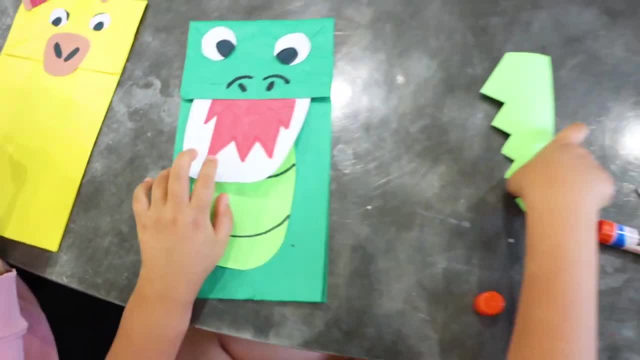 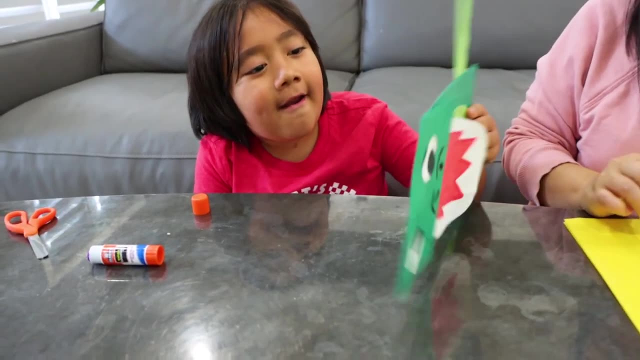 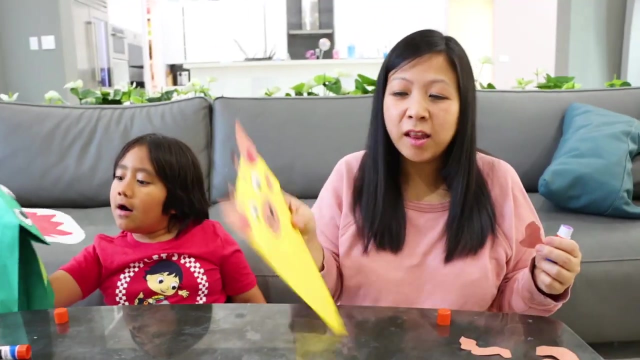 Okay, I'm putting on the body And now the tail. Okay, I got the tail. Now I'm done, And I'm almost done. All I'm missing left is a few spots, So I'm just going to put spots around my giraffe. 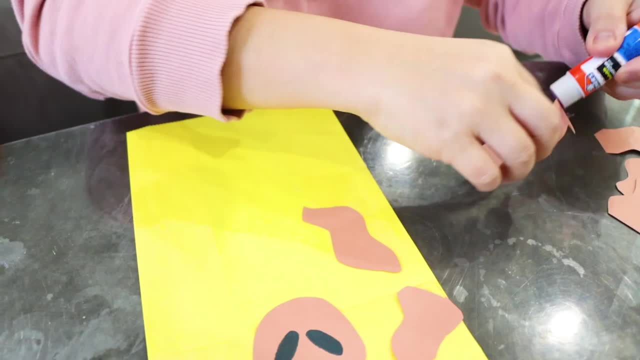 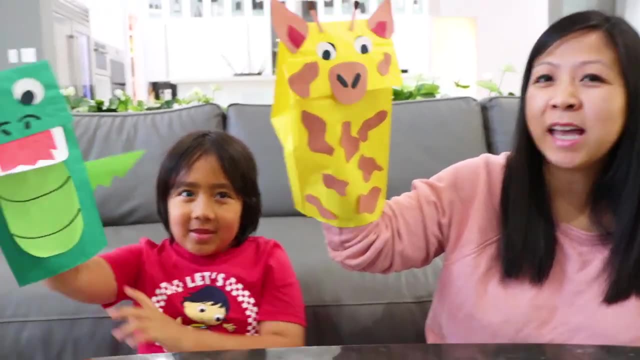 Like so. Ah, not yet I'm not ready. Alright, a few spots. You can randomly put it anywhere you like. Alright, I'm done. Hi guys, I'm Gio the giraffe And I'm Ellie the alligator. 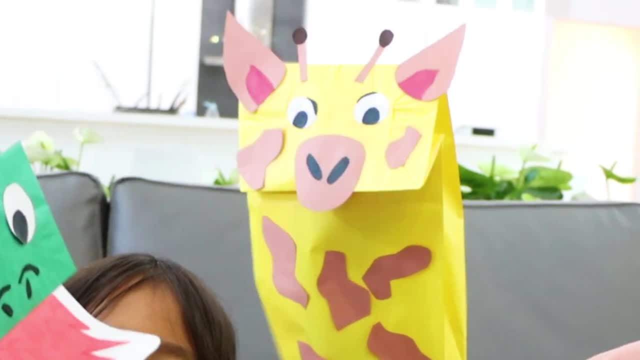 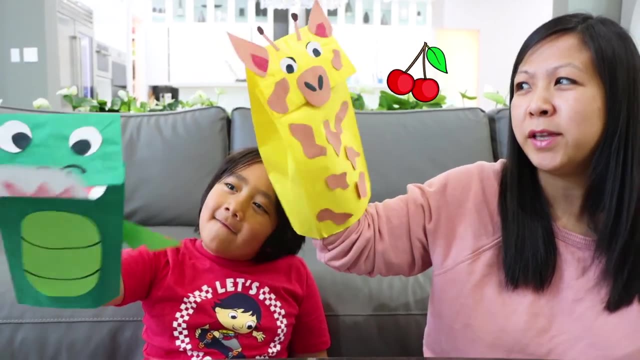 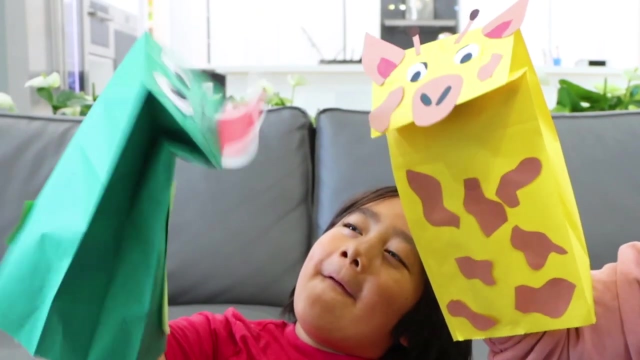 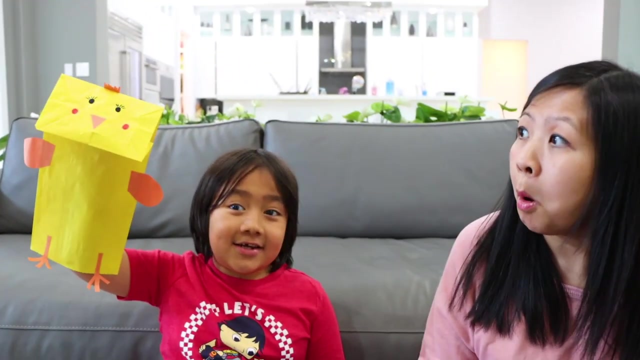 Oh, Ellie, I'm hungry. Do you have some leaves for me? No, What about cherries? Wait, do giraffes eat cherries? No, Oh right, Can we become friends? Yes, Yay, Okay, and you can make some more like this: 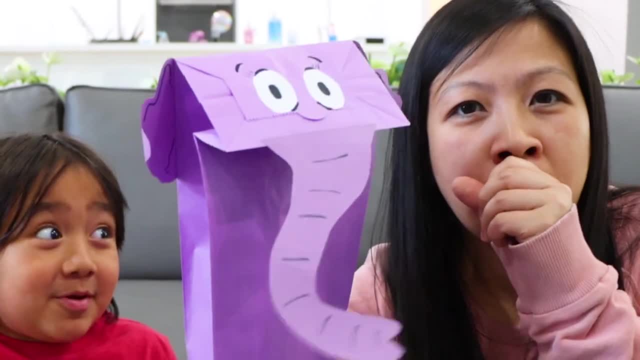 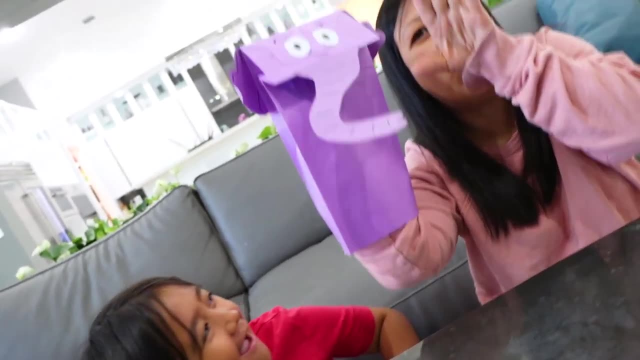 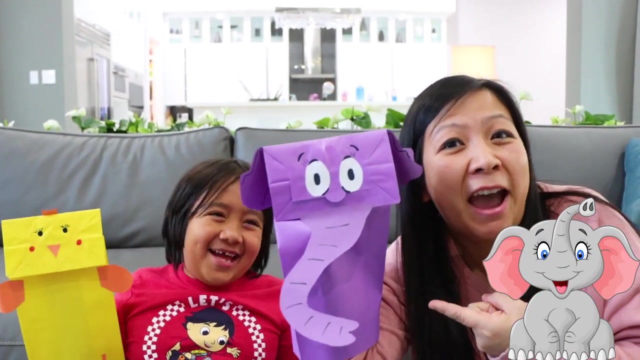 Cheep, cheep, cheep, Cheep, cheep, cheep. What animal is this? Did you guys guess it? That was my elephant, That was my elephant sound And Ryan, yours was A chicken. Okay, guys, guess this one. 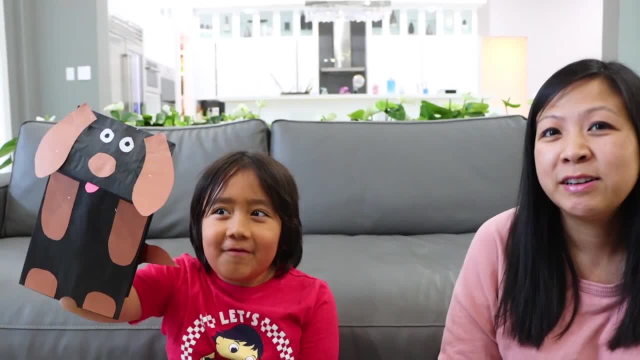 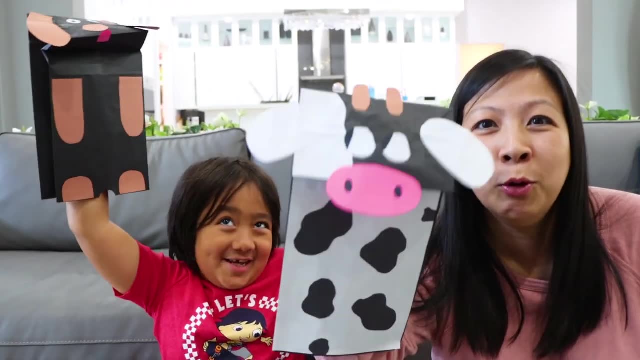 First, First, first, Guess mine, Moo Moo. I wonder what that one is. Do you have some grass? I eat grass. You said you could do good at that. That's very bad, Is it bad? Yeah, Moo. 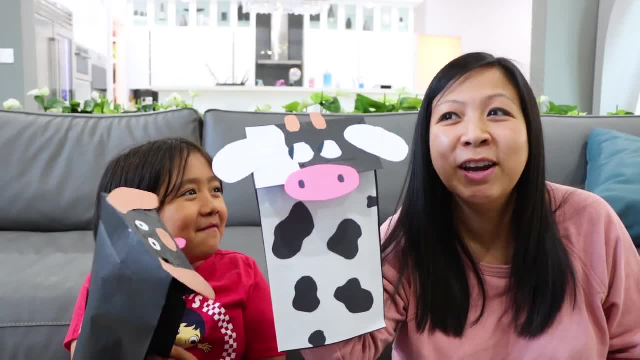 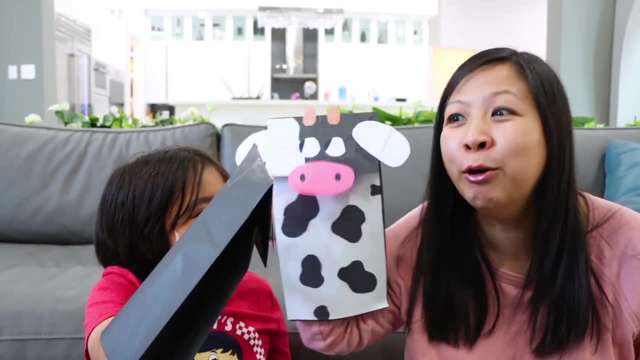 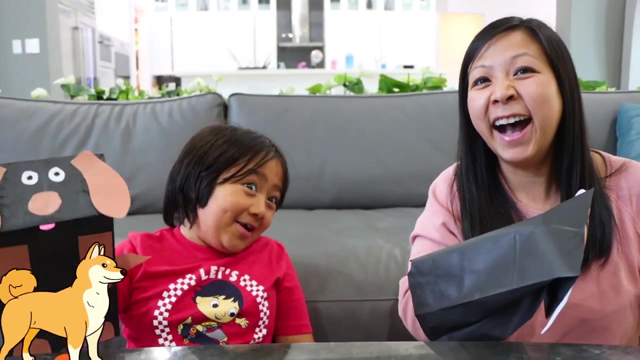 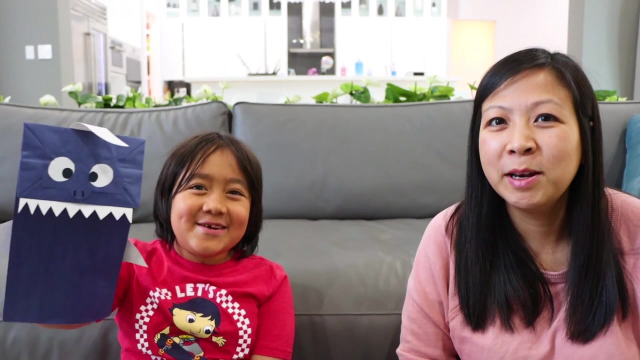 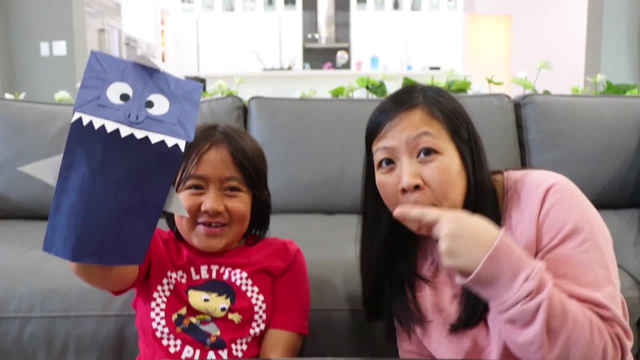 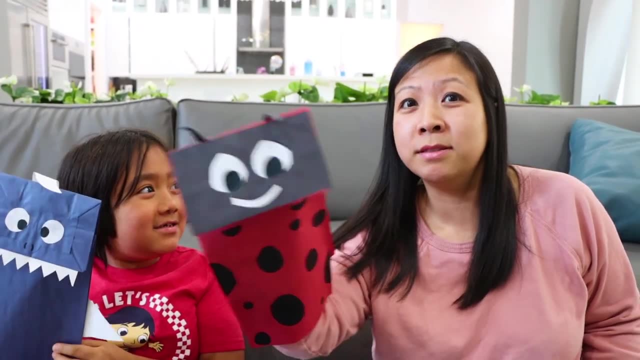 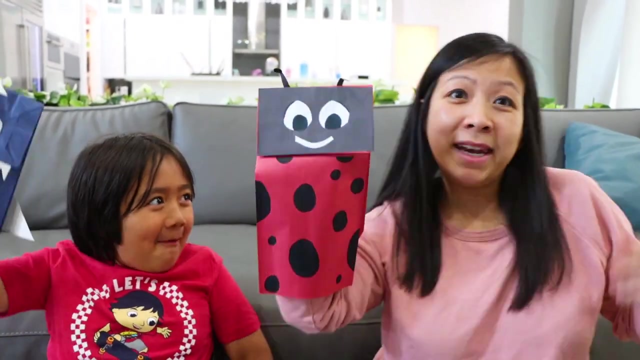 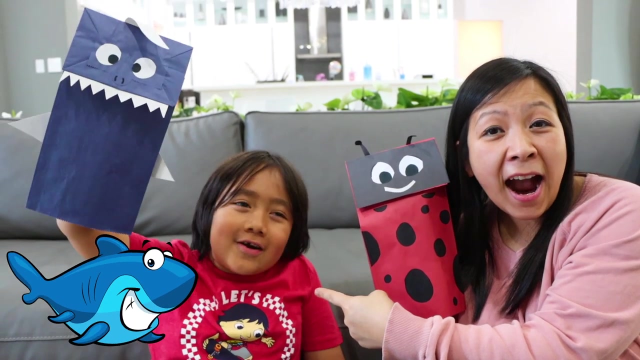 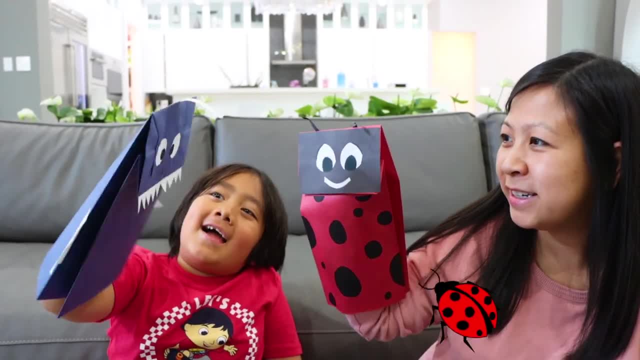 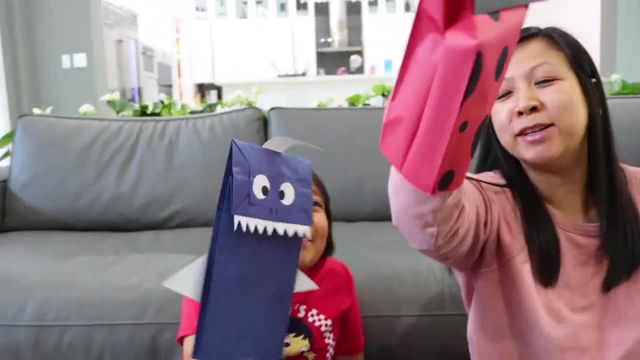 And Mommy is a ladybug. Oh hey, shark, Hi, Are you a baby? Ah no, I'm flying away, I'm flying away. Sharks can't fly, Sharks can't fly. Last one, guys, Which one is this? 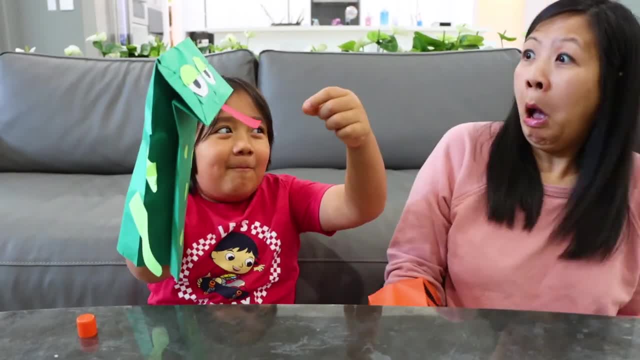 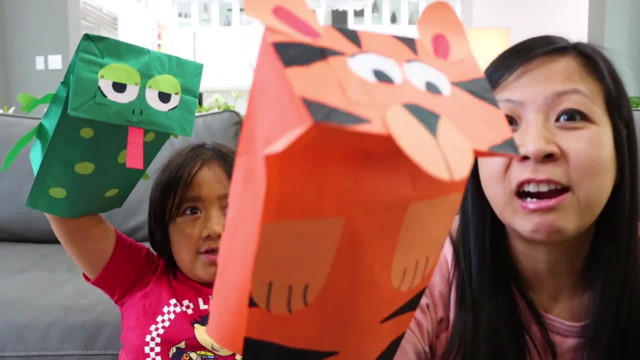 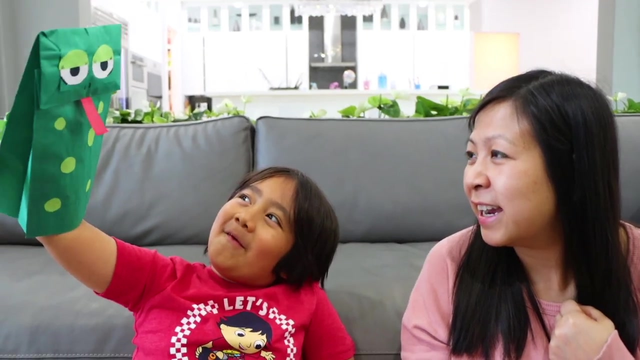 Ribbit, ribbit, ribbit. Oh, poor fly, And you guys know this one. Grr, grr. Is that the right sound? Grr, Did you guys guess? Ryan's? It is a frog, if you didn't know. 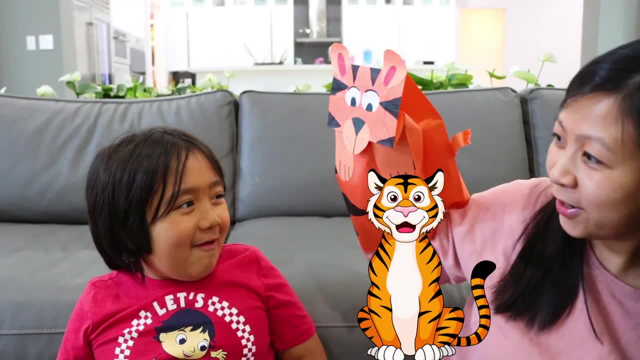 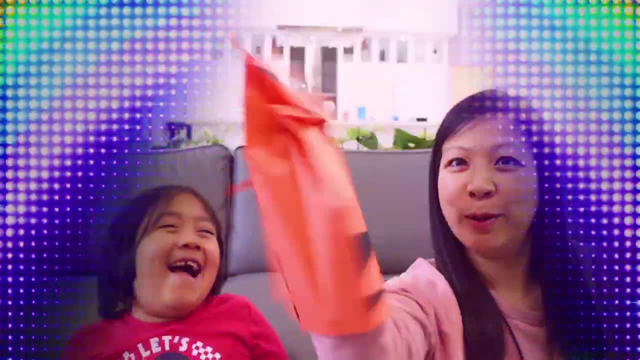 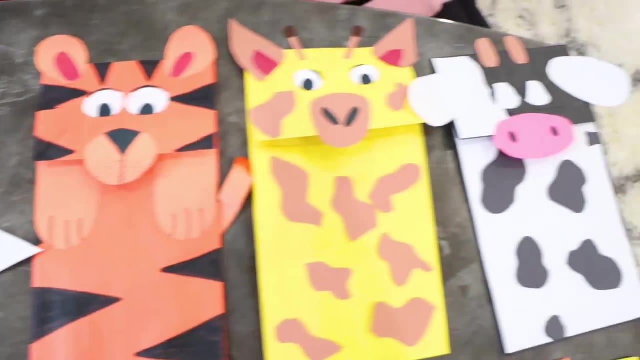 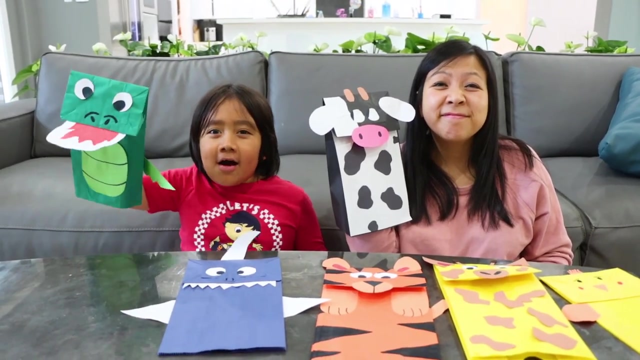 And mine is Tutu the tiger, Because I like to dance with an invisible Tutu. Thank you for watching our easy do-it-yourself Animal paper bag. And which one do you like? Okay, guys, Thank you for watching our video. 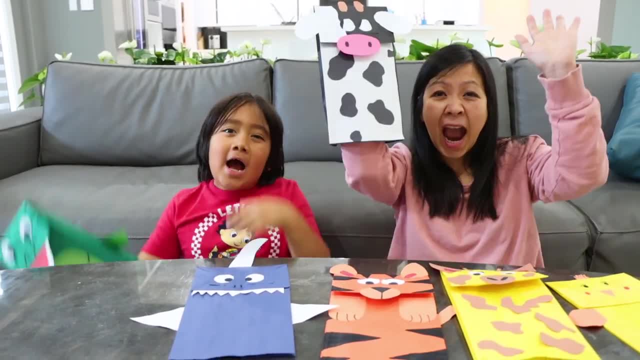 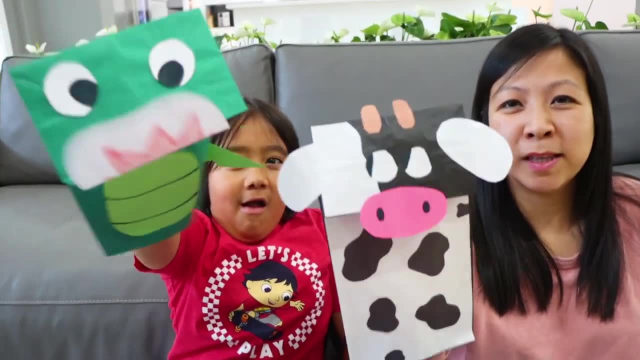 Bye, Remember. always stay happy and rise up. Bye, Oh, alligator says bye, And then my cow says bye too, Moo, Bye, Bye, Bye. Okay, guys, Today, me and Mommy are going to try to paint. 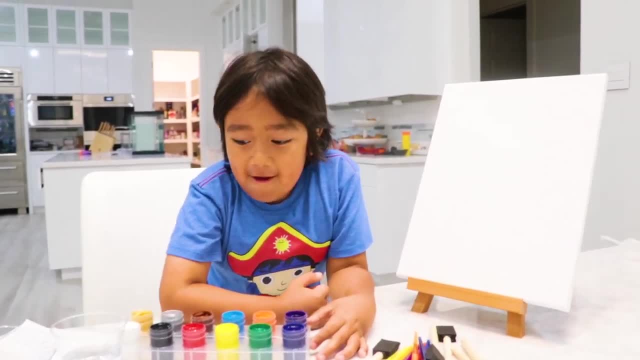 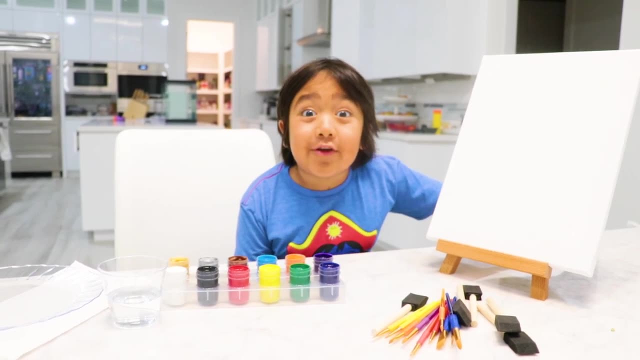 Even Each other. Yeah, Ryan's going to try to paint me And then I'm going to try to paint Ryan When Daddy goes home. he's going to decide the winner And you guys can decide the winner. Okay, All right, let's get started. 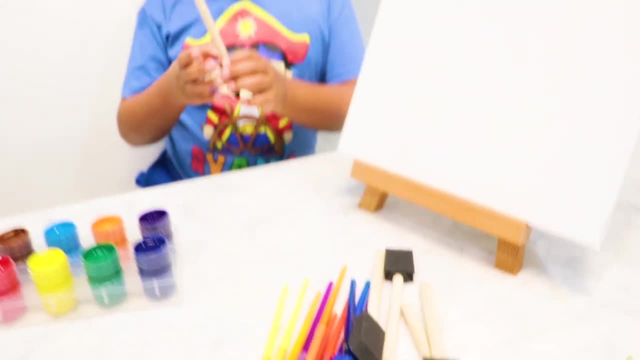 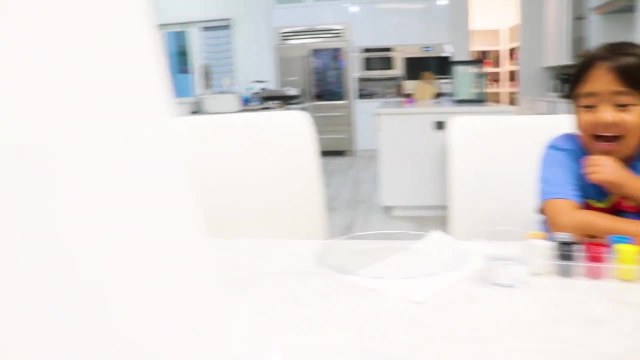 So we have our paint here, our paint brush here. Let's get started. Let's see here- I don't know how to start. I need peach because Mommy's tan- Yeah, we don't have peach, so we're going to just paint. 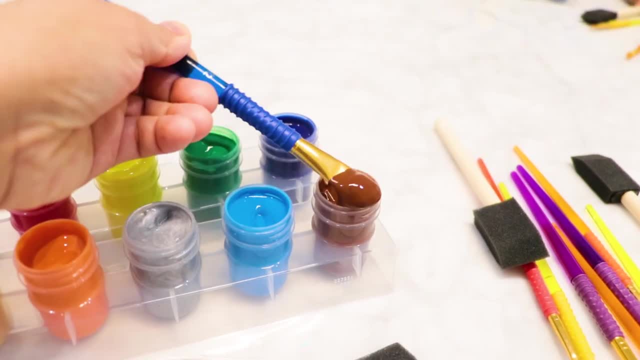 Okay, We're going to get a little bit of brown- Is that how you make peach, Maybe, See? And then a little bit of white, And then, I guess, just going to just mix them together. Okay, what about some orange? 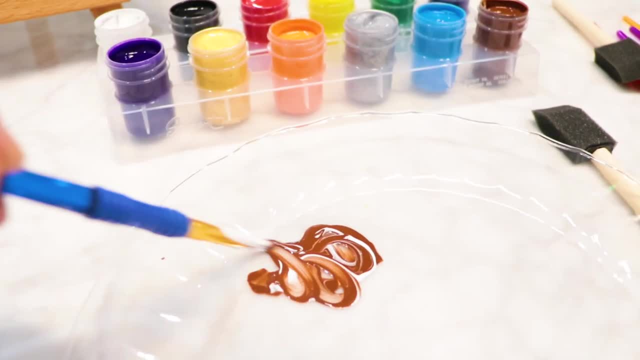 Whoa, this is not looking like peach guys. How are you doing Good? All right, I'm going to use black here to draw the outline. It looks like a pencil Surface. pencil of the world, Mommy's hair. 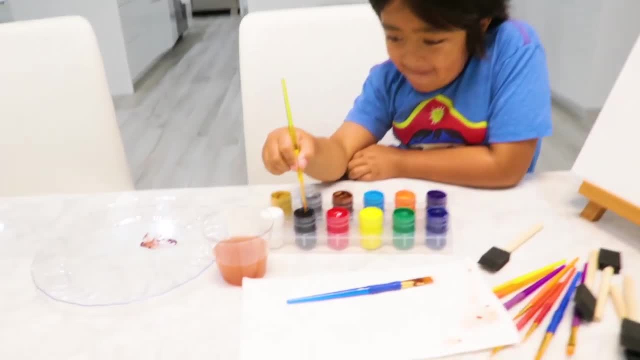 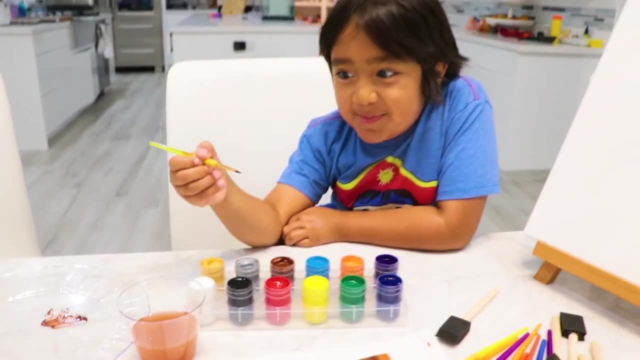 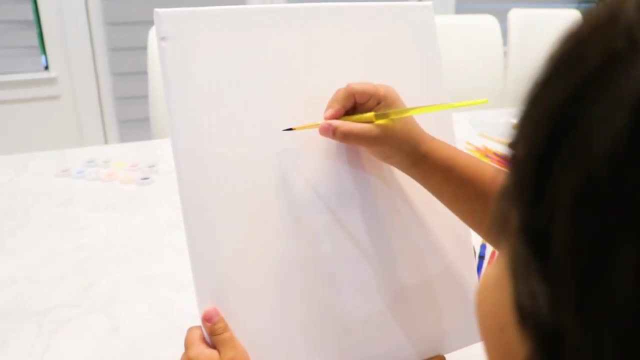 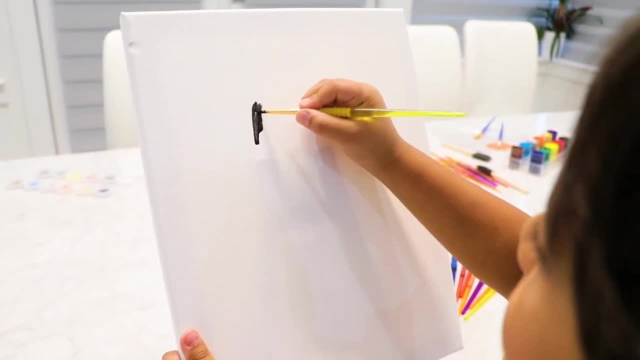 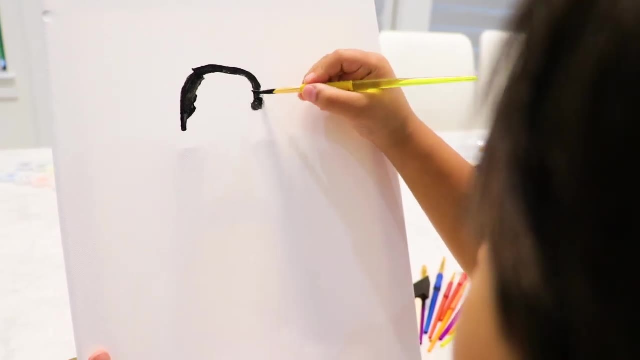 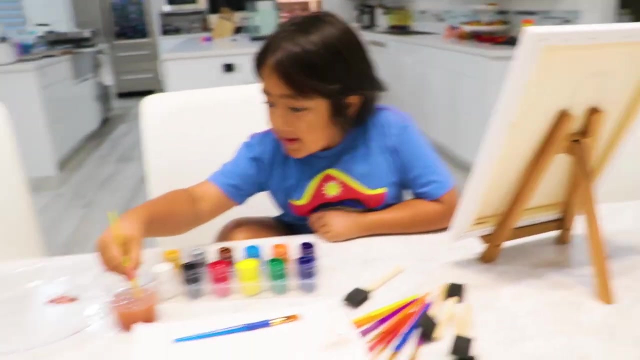 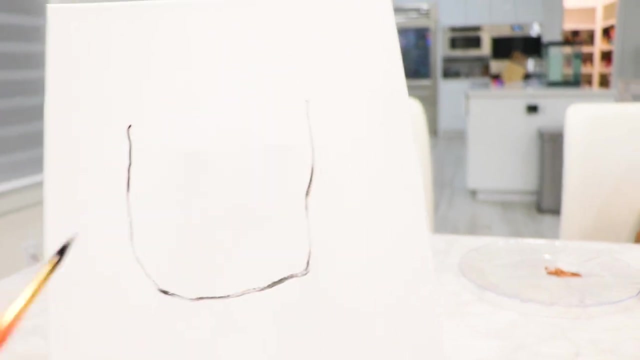 While Ryan's drawing me over there. I want to draw Ryan. He's trying to take him out. I'm going to draw Ryan. I want to draw Ryan. so Ryan, right there. You just girl. How are we what? Nothing, this is your face so far. 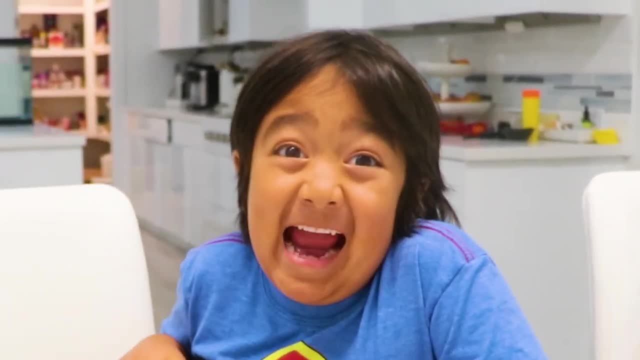 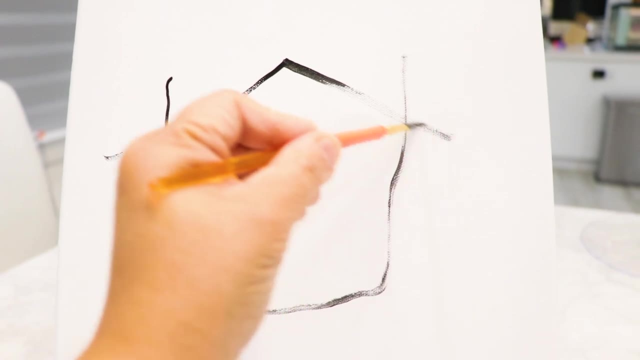 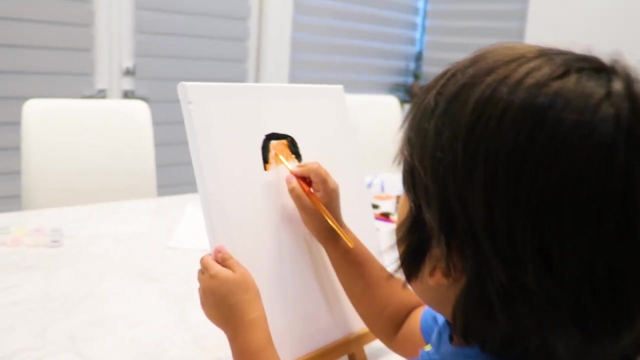 What you think. So Ryan likes it so far. approval, Do I? How am I gonna use peach, though? Oh, I think you need yellow, Maybe. Okay, this is Ryan's still. Whoa, is that my face? Yeah. 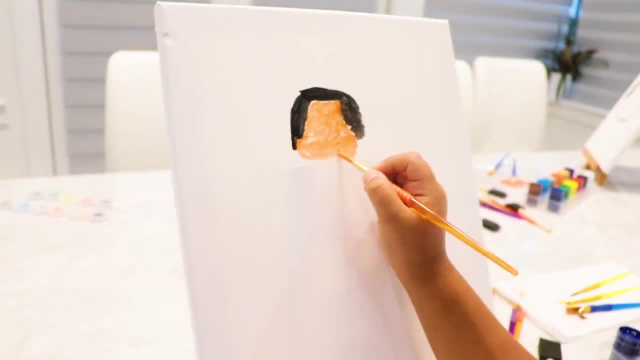 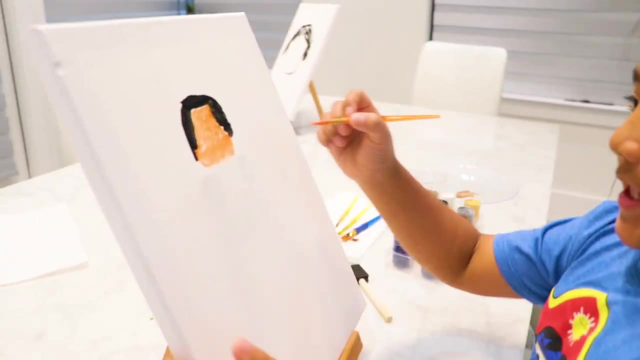 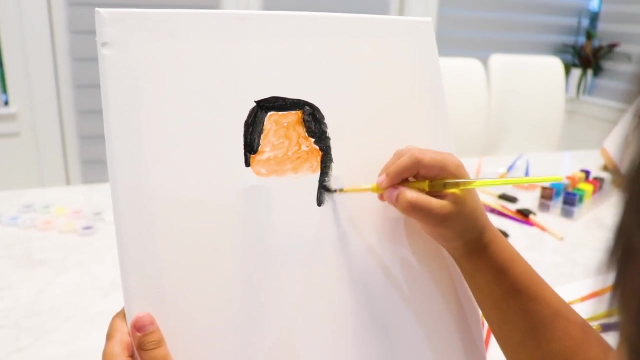 I'm making it bigger. Whoa, Ryan. Why am I orange? Because that's all I have. Yeah, Good job, though Sharp as it gets. Ah, Oh, I'm making my long hair, Ooh, fancy. Okay, Ryan's getting to my eyes. 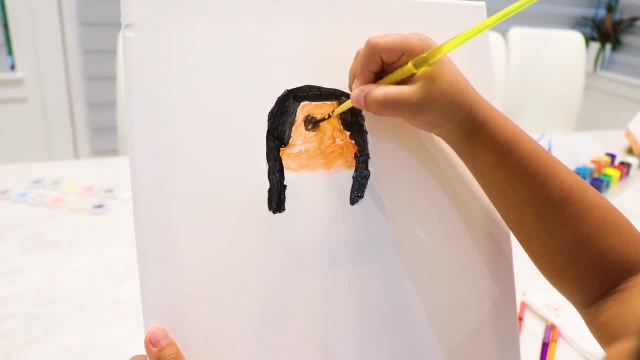 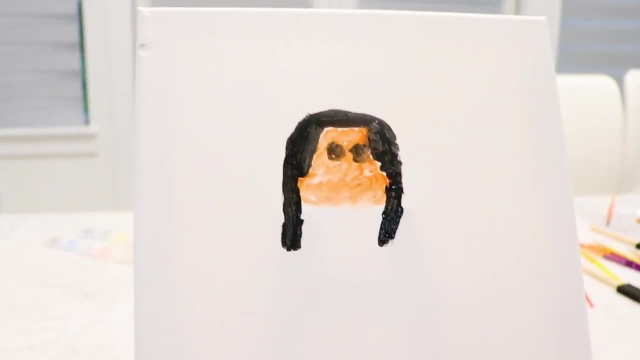 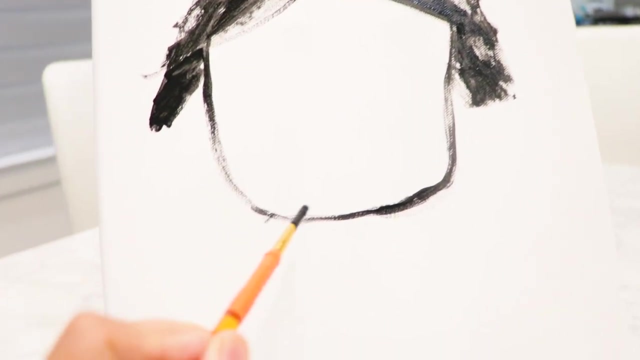 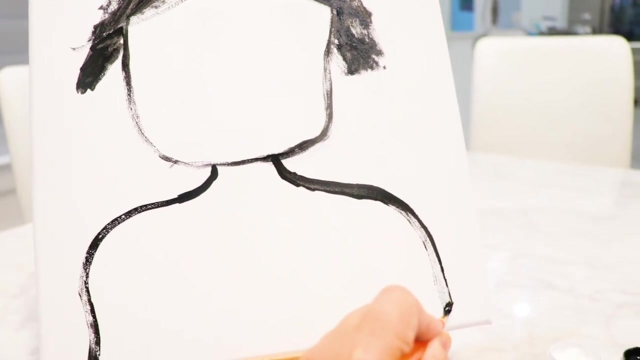 Oh, this is harder than I thought it would be. Giant eyes- Whoa, does that look like me? Okay, that's what I have so far. I'm gonna continue here with Ryan's neck. What are you laughing about? Okay, guys, why is Ryan laughing? 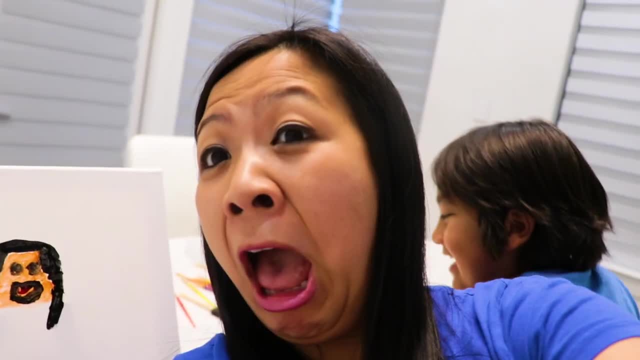 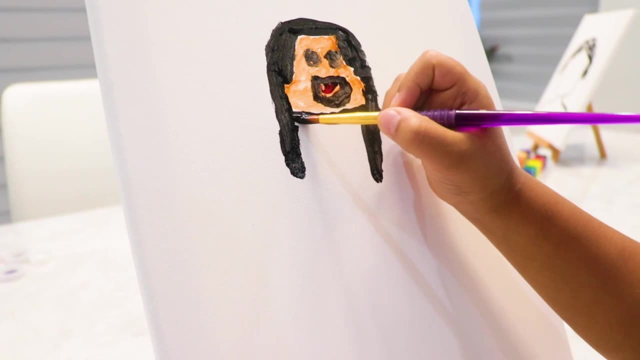 Whoa, what is that Ryan? What is that Ryan, Ryan? Eh, Ah, It's a mouth. It's a mouth, Huh, It's a mouth. Whoa, Ryan drew me with huge neck. Whoa. 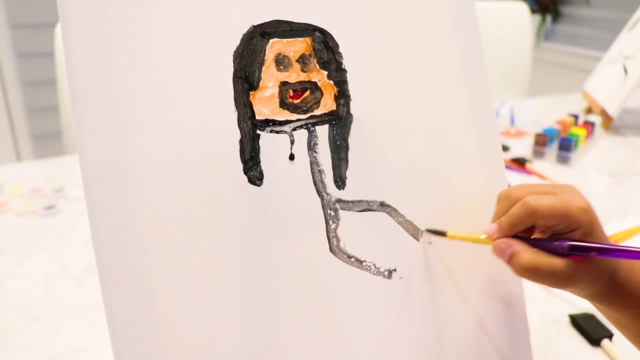 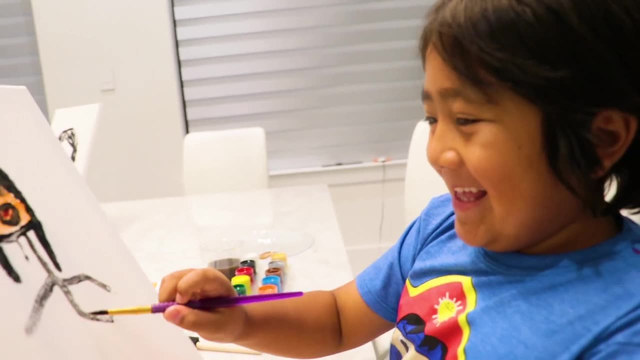 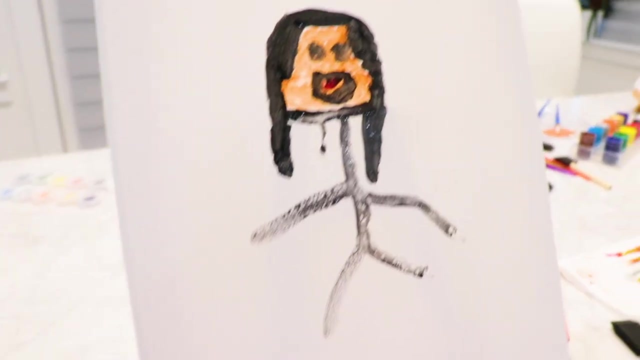 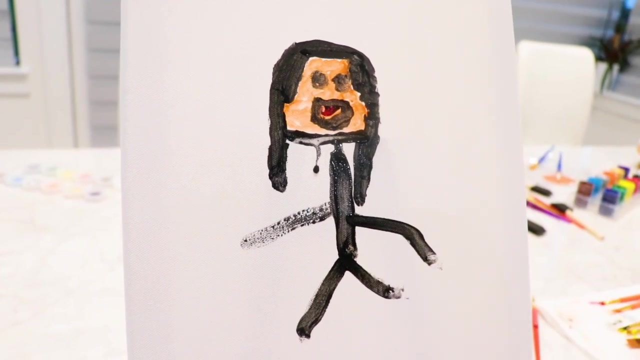 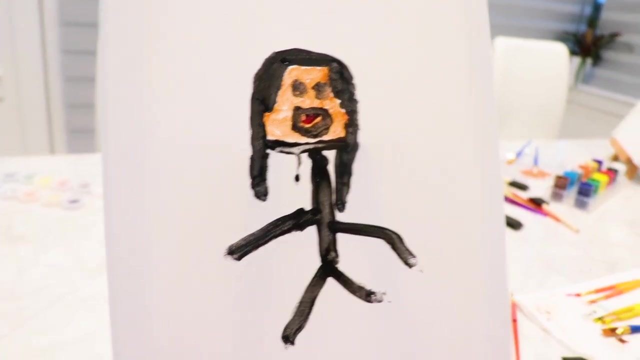 What is going on? Get your arm. Well, I worked out What is going on. Oh, a stick figure. I see Ya stood and I look like mommy. You look like a monster, mommy. I'm not done yet. So while Ryan's continuing, I'm gonna do mine continuing. 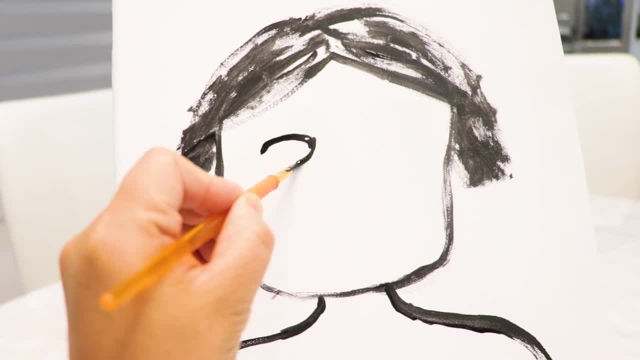 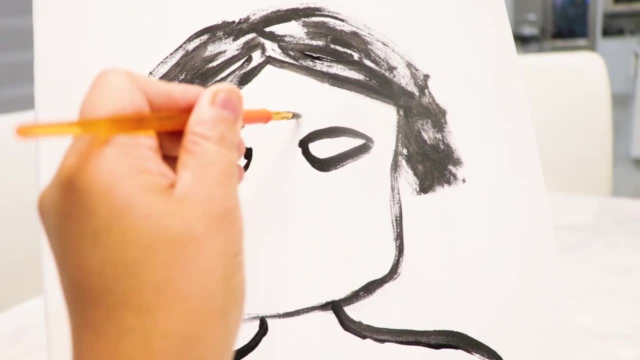 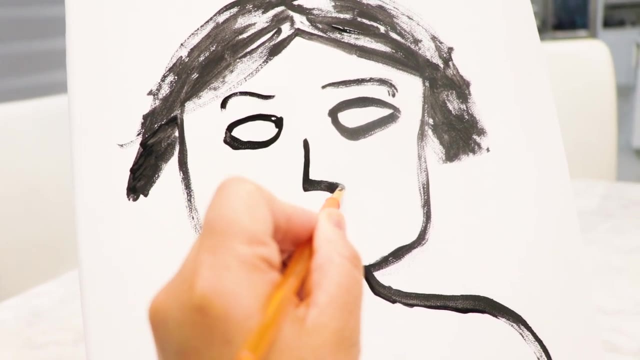 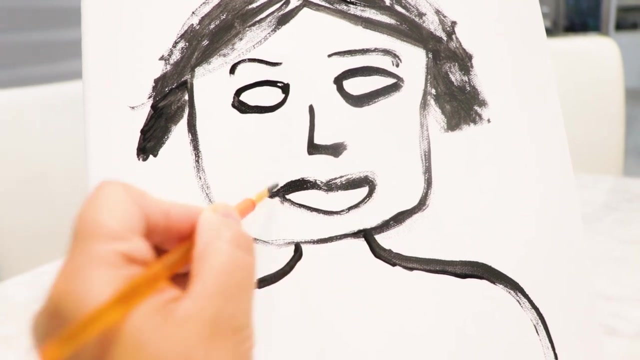 I'm gonna dry Ryan's eyes, Okay, Okay, Ready Ryan's other eyes, Eyebrows- I like how they're not even even. They're not even even. Yeah, The nose And the mouth. Can I give you a hint of what I'm drawing? Uh huh. 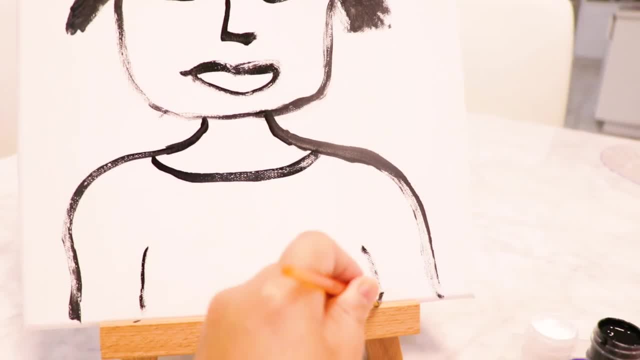 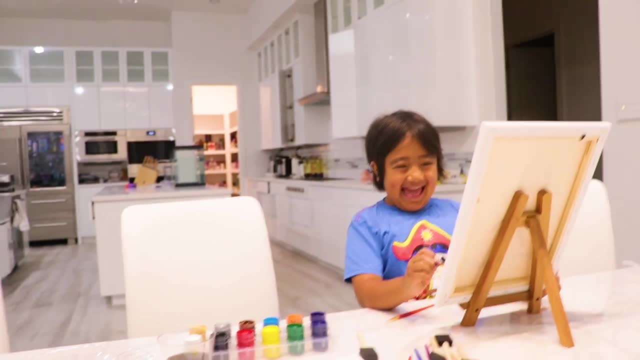 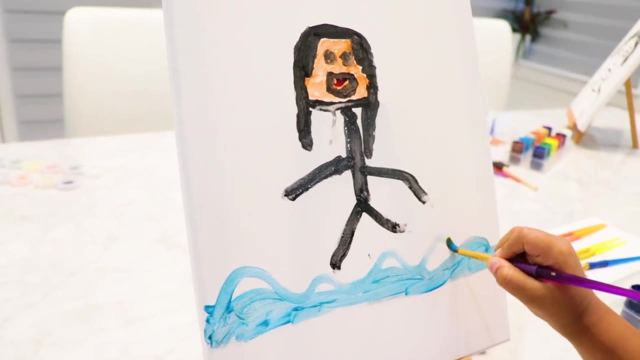 You have to be waterproof. Whoa, I'm a mermaid. No, Okay, this is Ryan continuing. Oh, am I in water? What's going on? You're falling, Oh, no, Am I a zombie? mommy falling from the sky. 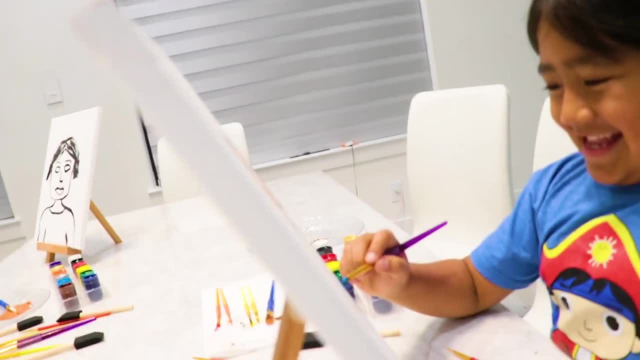 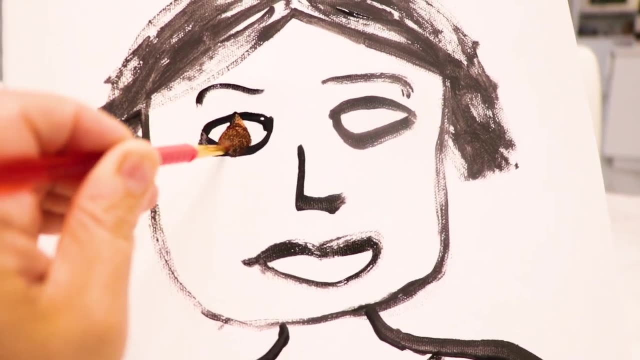 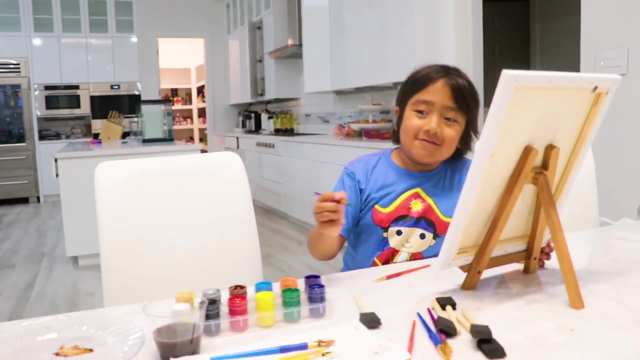 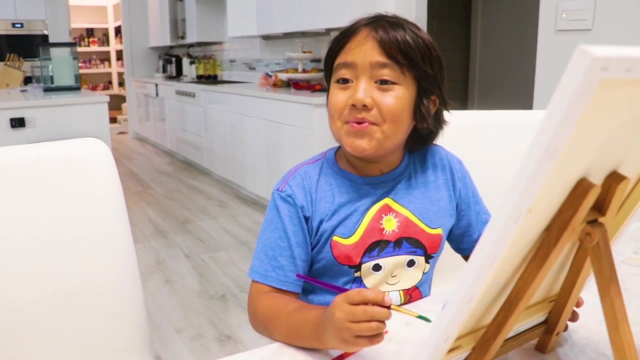 What is going on? Ryan Cute, Okay, drawing Ryan's eyes. You want to see what I have so far. That looks pretty good. What do you think It looks pretty good? Yay or nay? Yay for the. 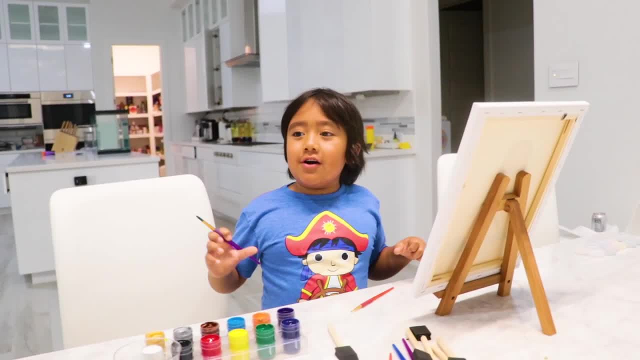 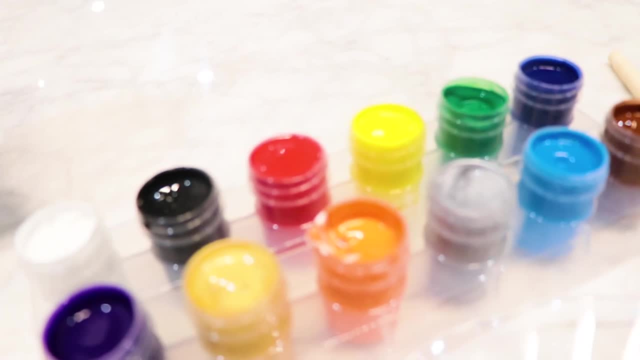 other, like the parts, like the shirt and the hair, but nay, for the head. Okay, I'm going to give Ryan. is it weird to give Ryan red lips? No, no, no, no, no, no. 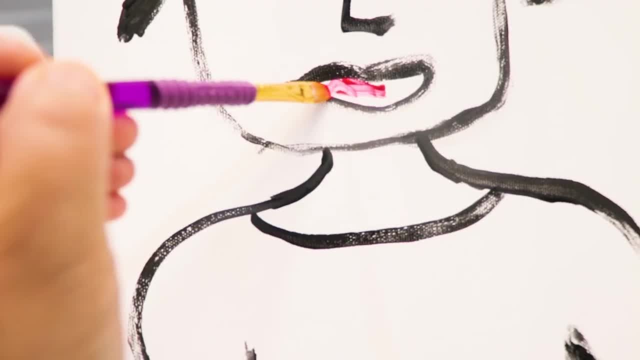 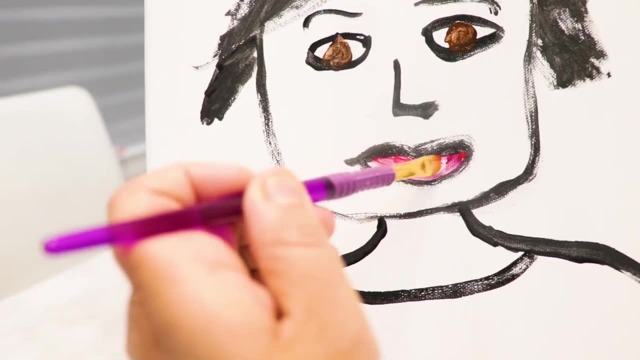 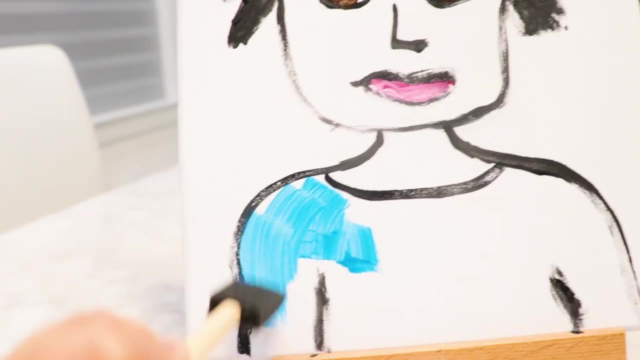 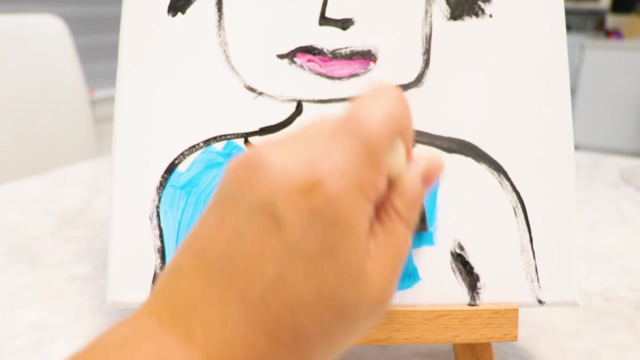 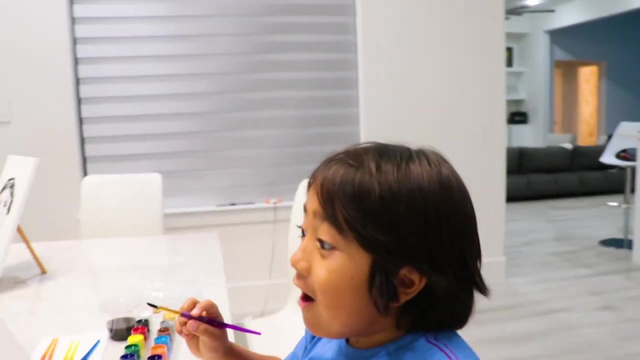 What Red lip? No, No, Too late. I can make it white a little bit Ryan's lips. I'm going to give him a blue shirt, since he's wearing a blue shirt right now. Yeah, What happened? It's getting messed up. What is that on my head? 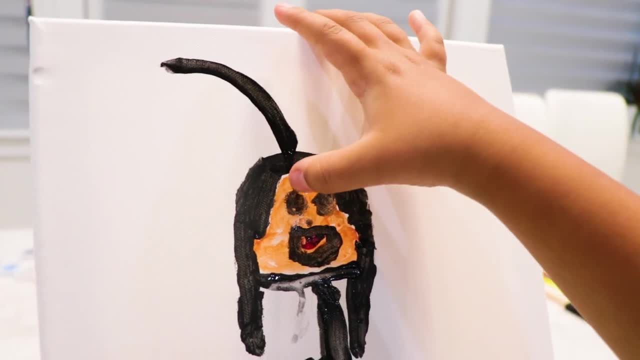 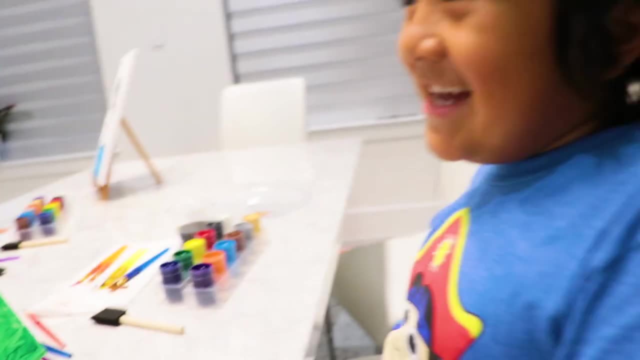 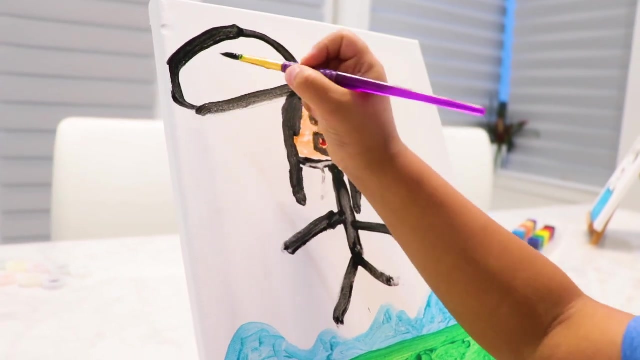 What is this? It's getting messed up. What is going on? What is that? Do I have an antenna? No, It's okay, I'm in the air, you guys? What is that? I'm so confused. what he's drawing? Do you guys know what he's? 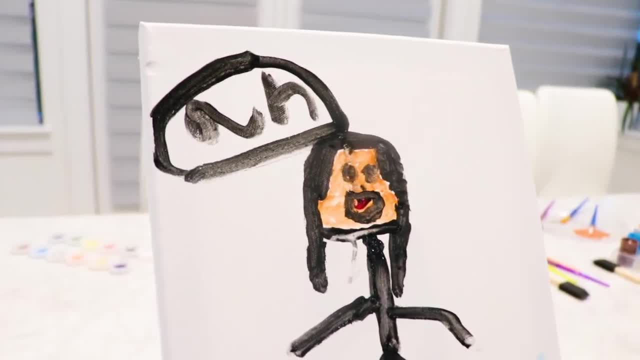 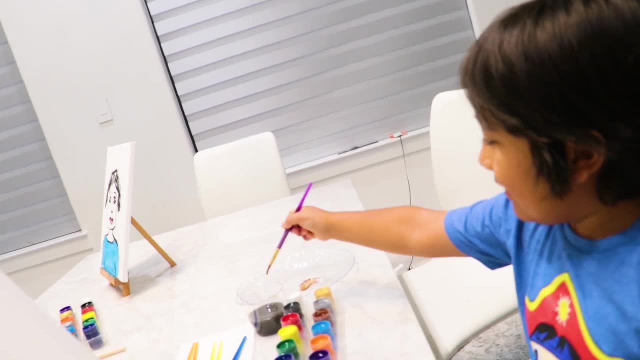 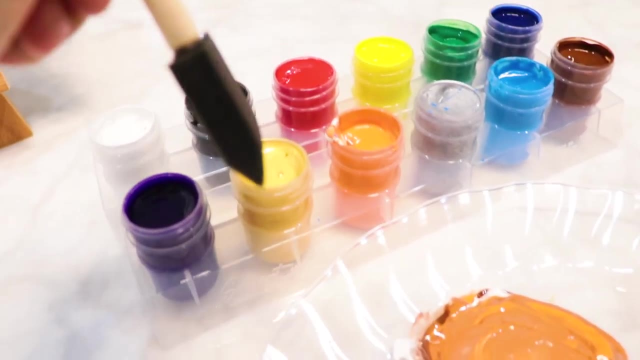 drawing. Oh, a bubble. Am I falling? Is that why, Ryan? Yeah, That looks pretty good, Ryan. Okay guys, so I was going to use this, but it doesn't look very good. What if I color Ryan's gold? 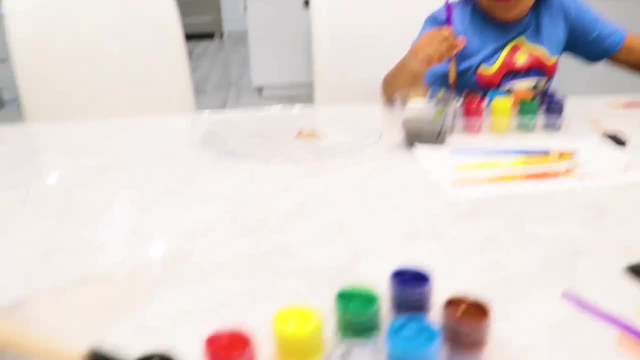 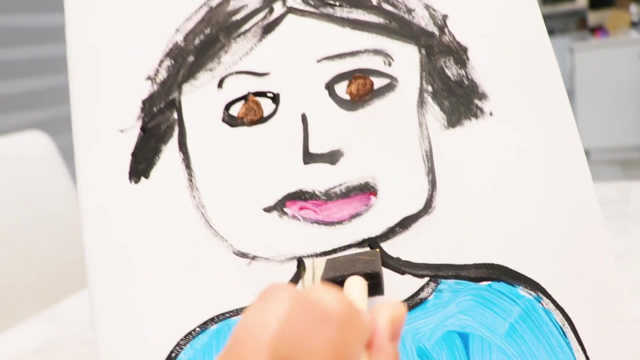 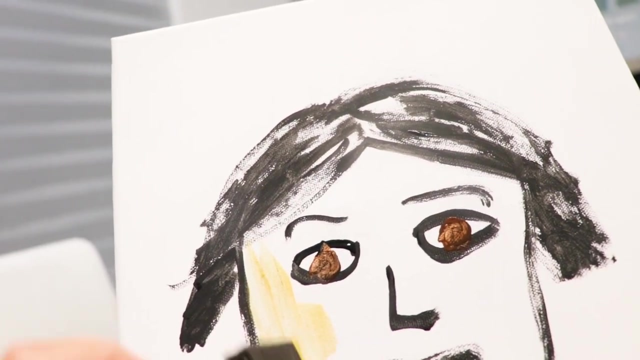 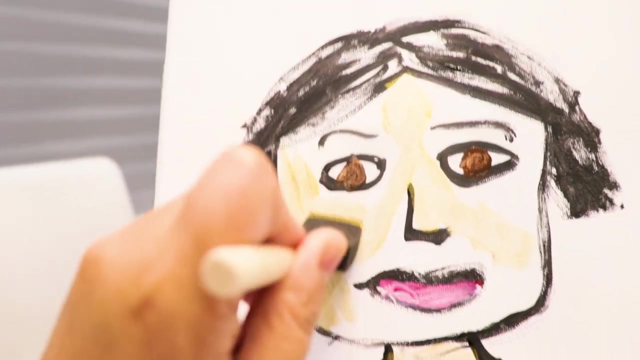 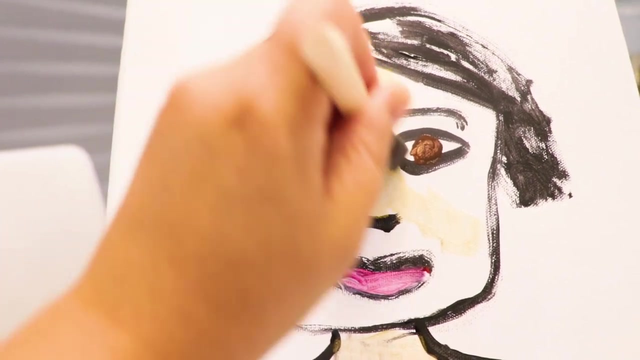 Gold, Ryan Gold. Let's see what it looks like here. Ah, it's smearing. I should have let it dry a little bit more. I should have colored the face first before I colored the eyes and stuff. Yeah What. 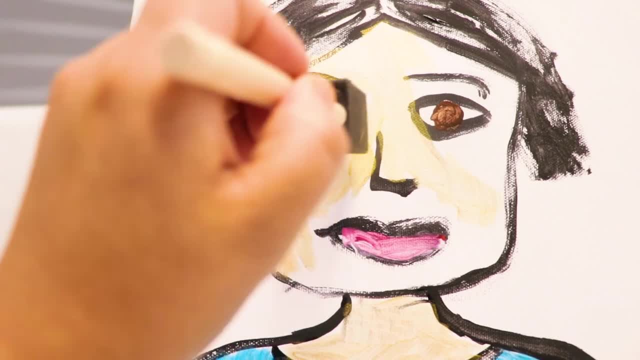 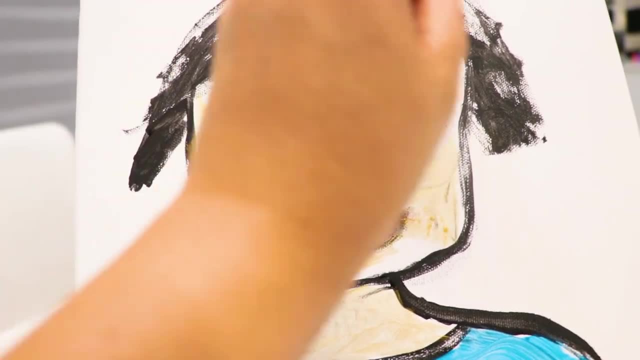 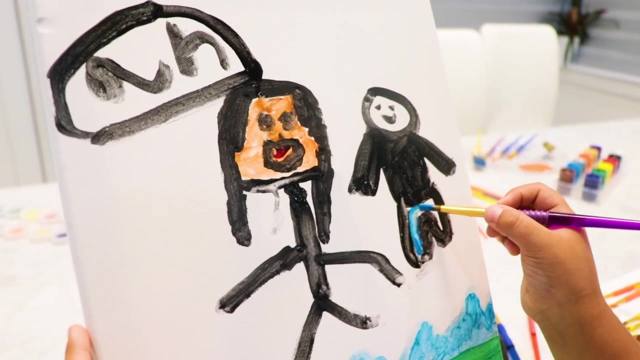 Now it's smearing. Okay, guys, what do you guys think so far? Alright, this is Ryan. I don't know why he's drawing a random person there. Is that you, Ryan? No, Is that Emma? Is that Kate? No, 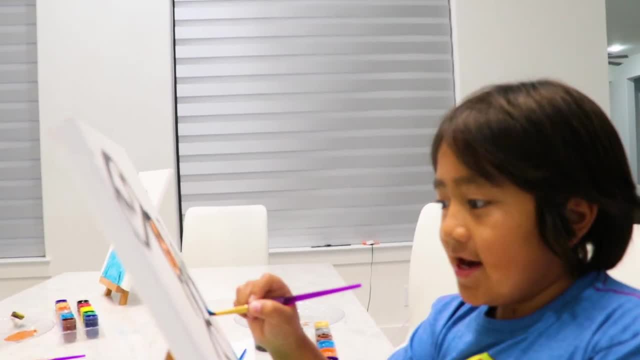 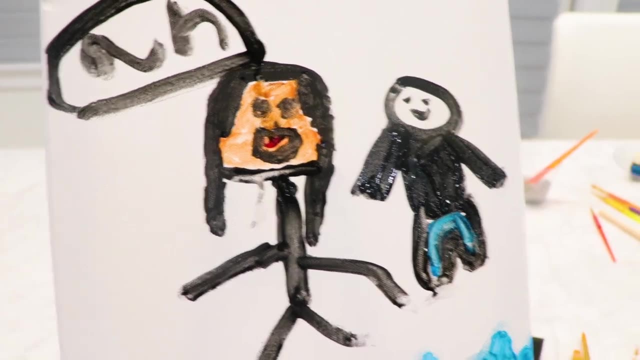 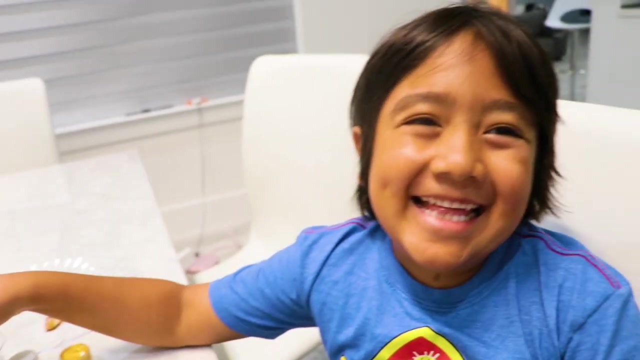 It's not daddy either. Is it my sister? No, No, Just a random little girl. I don't know if it's a girl or a boy, It's a stick figure. Actually, that stick figure looks better than you, Hey. Hey. 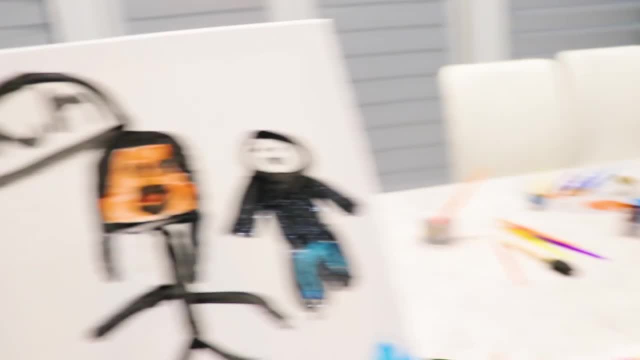 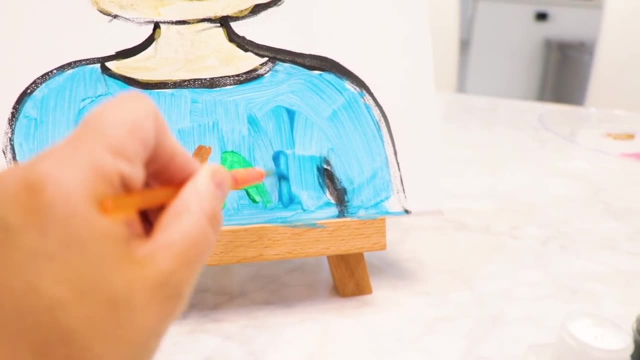 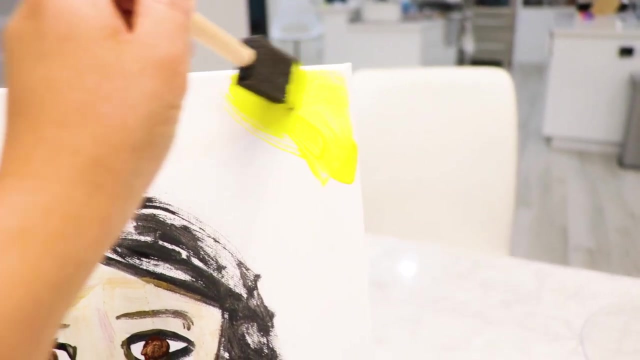 But I put less effort into it. It is cuter. Hey, Okay, and then M, Oh, but it's blue, so it's kind of the same. That's not good. Okay, guys, now I'm drawing the sun because Ryan's logo is a sun. 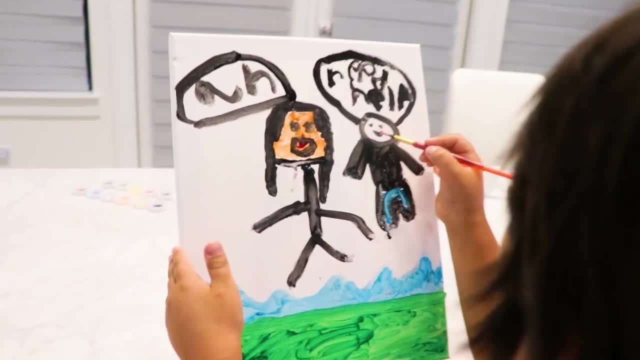 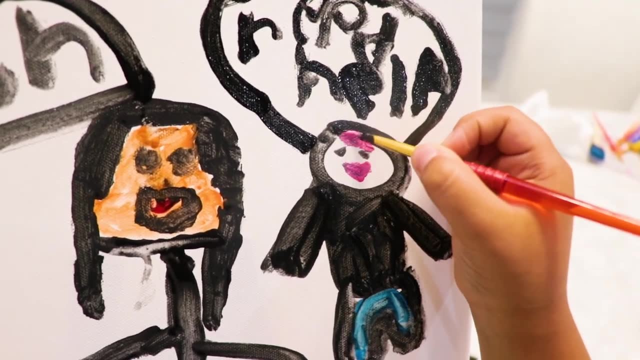 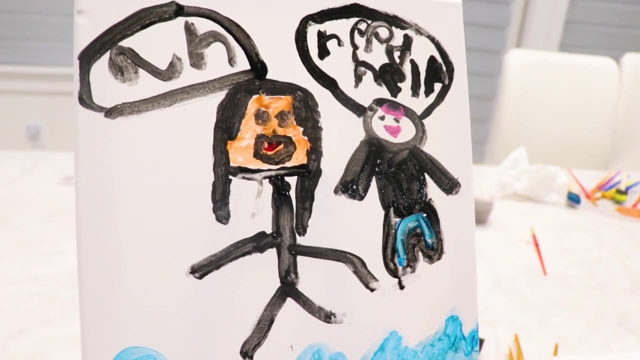 Okay, there it is, Ryan. The little girl needs help. Oh, so my rescue person is helping the little girl- A nice zombie mommy. No, the girl's saying: do you need help? Oh, she's trying to rescue me. 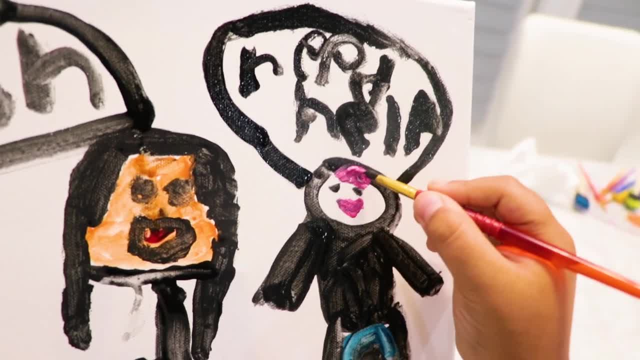 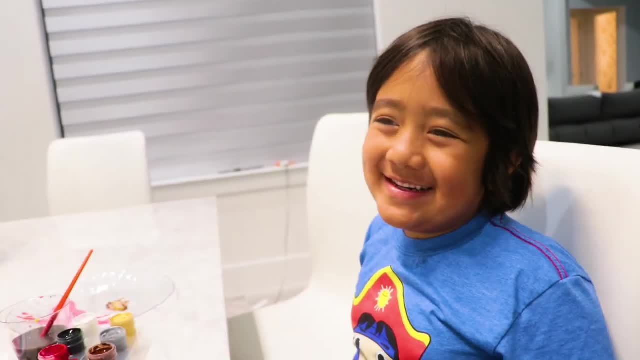 Got it. I do need help. What are you drawing? Like a bow? Oh cute. It still looks better than you. This is your official drawing. You're done, Not yet, Not yet. How'd you get that color? 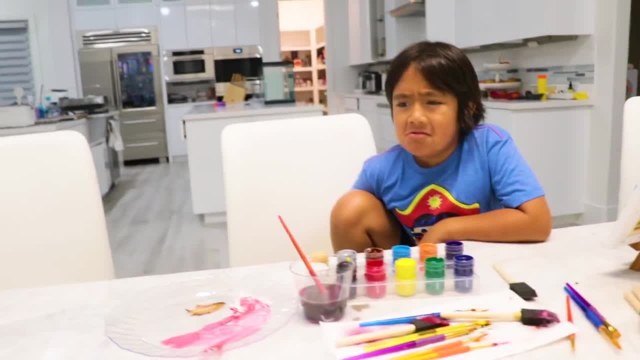 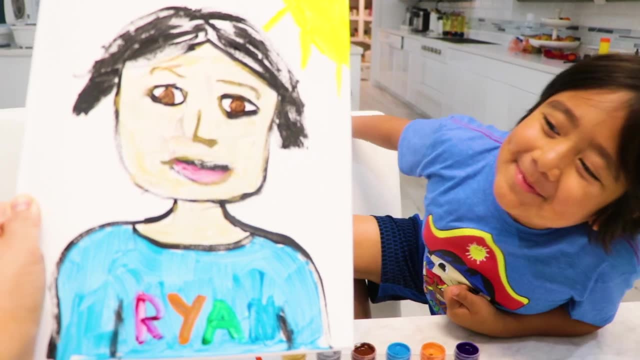 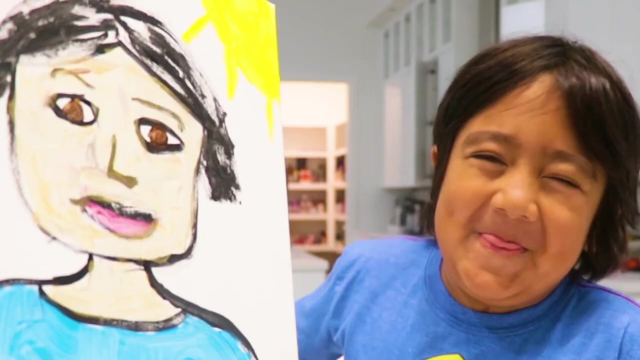 Okay, Ryan, So that's mine so far. What do you think? You don't think it looks like you. Look, it looks exactly like you. The skin color makes me look like a zombie. It looks exactly like you. No, No, You guys don't see the resemblance. 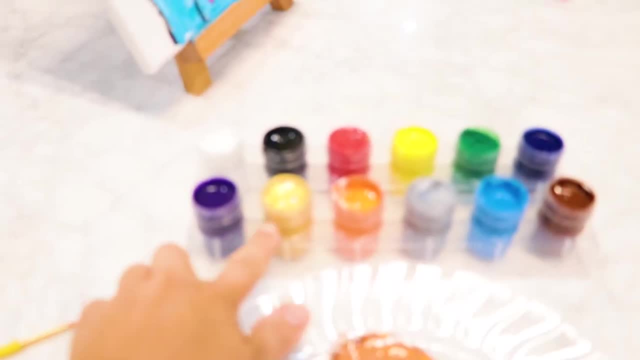 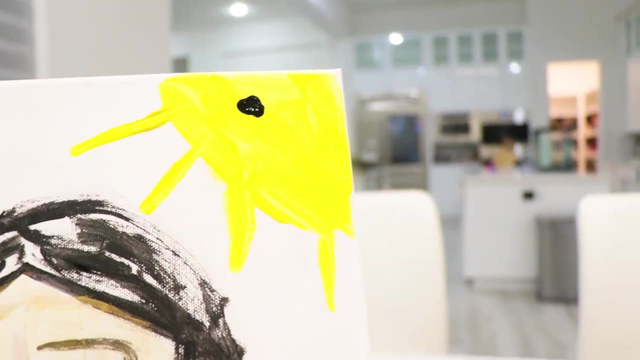 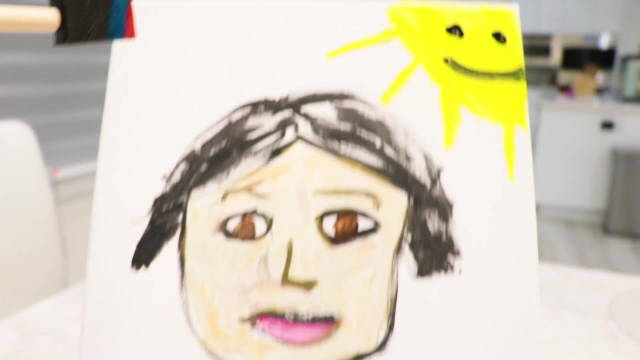 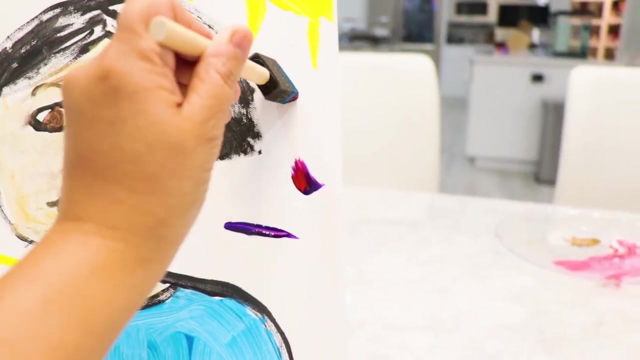 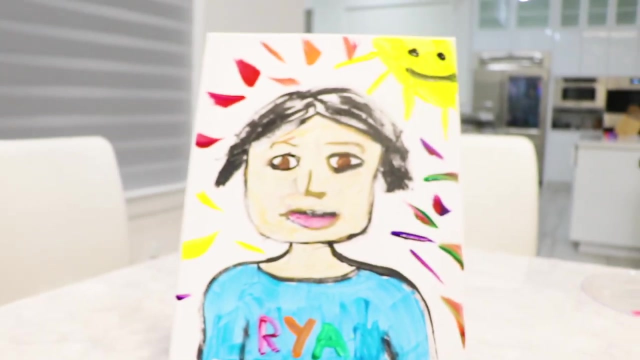 The skin color is because I used the gold. Okay, the sun needs a face, obviously, Okay, and I just like to just make it colorful. so I'm just gonna just make a whole bunch of lines, Just because. There, That is. 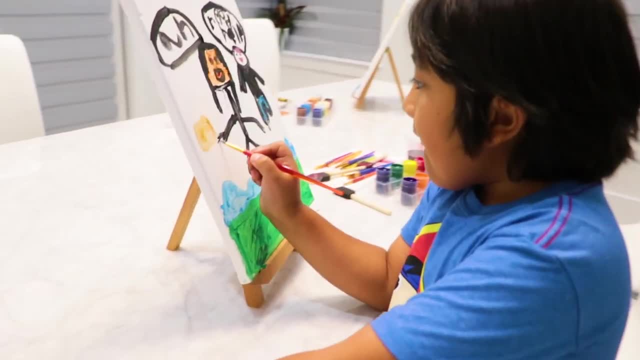 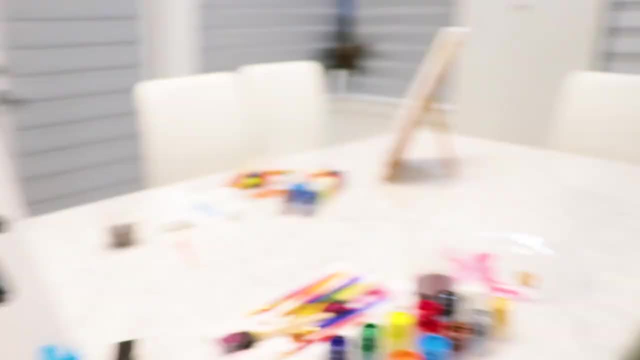 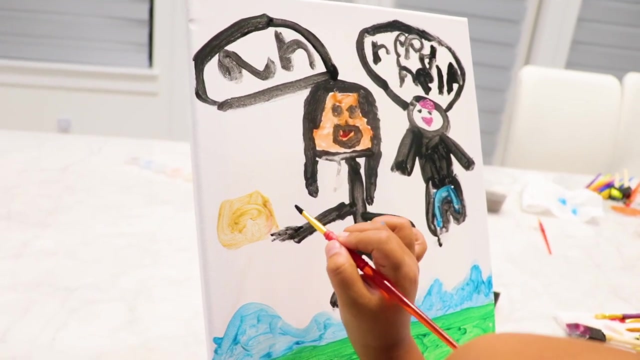 my drawing of Ryan. Okay, Ryan's still continuing. What is that? What am I holding? You're holding gold. Aww, Is that why gold is too heavy? Is that why I'm falling? Yeah, Or I can make you hold a weight, Okay. 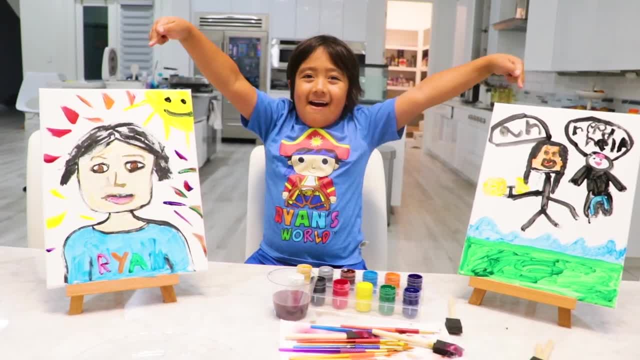 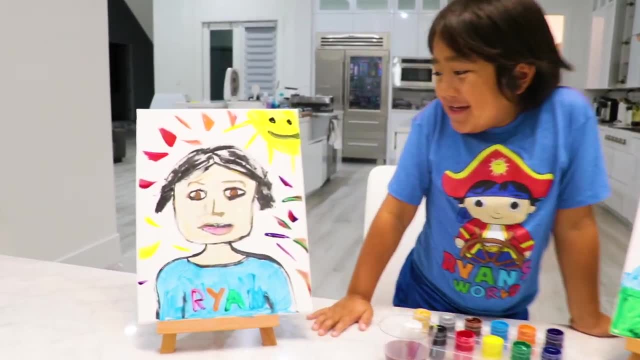 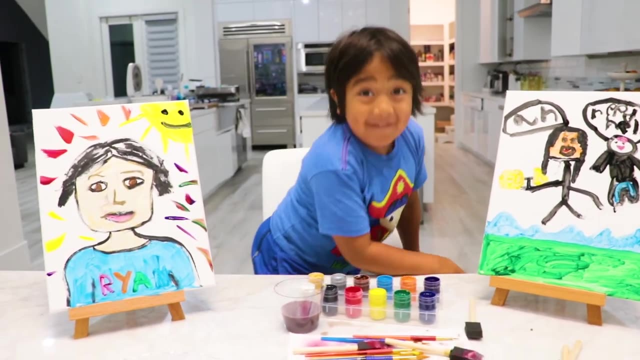 Okay, guys, here are ours. So this is Ryan drawing Mommy, and this is Mommy drawing Ryan. Mine looks like a zombie, Zombie Ryan. So now we gotta wait for Daddy to see which one's better Five minutes later. Okay, guys, Daddy's. 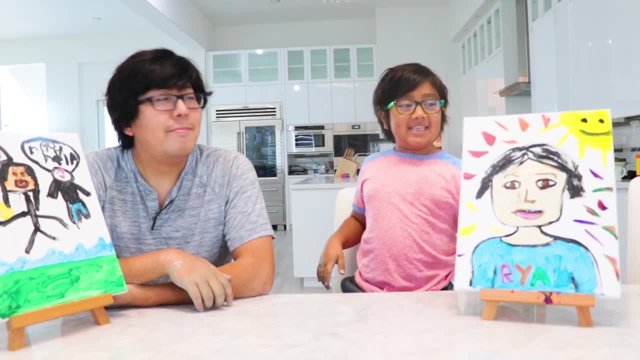 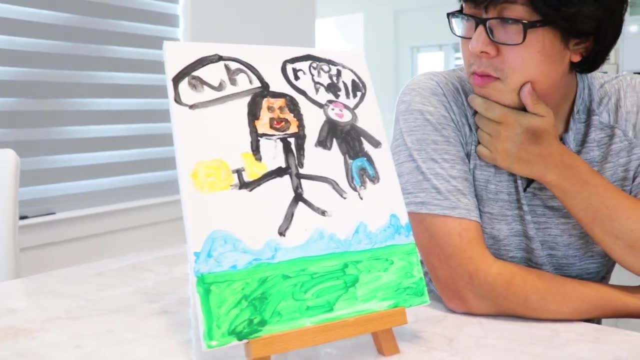 back and now Daddy's gonna see whose painting is better. Hmm, So this is Mommy's because Mommy drawed me and this is mine because I draw Mommy. Hmm, Interesting. So Mommy's falling because she's carrying. 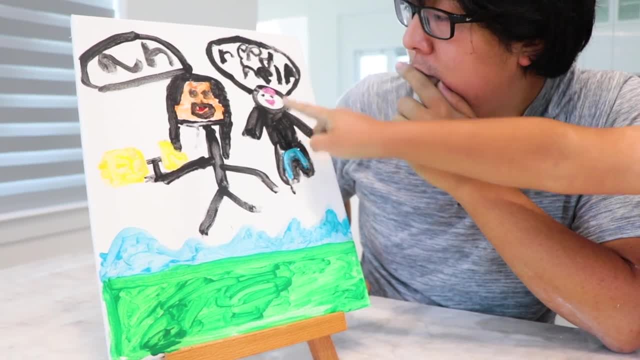 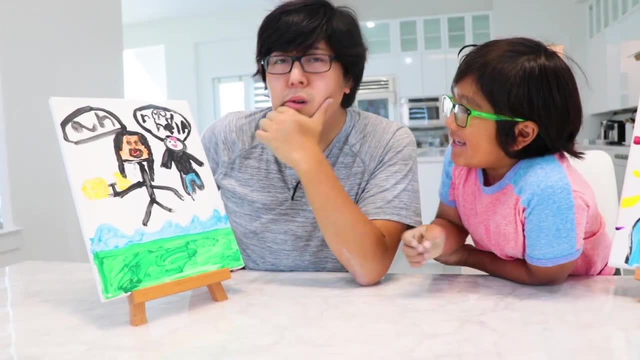 a gold weight and she's like: need help because she's super strong and then she can lift up the weight and then help Mommy. Oh, this is both of them, Mommy. Uh, no, This is a little girl. 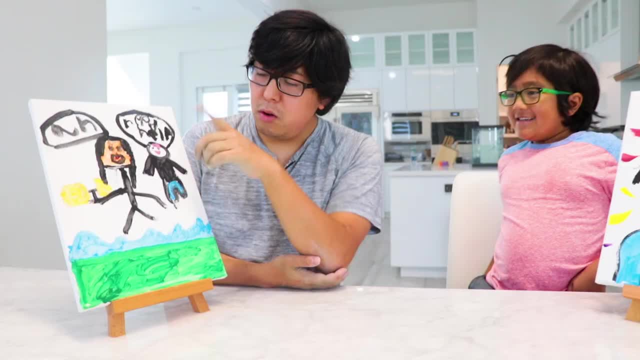 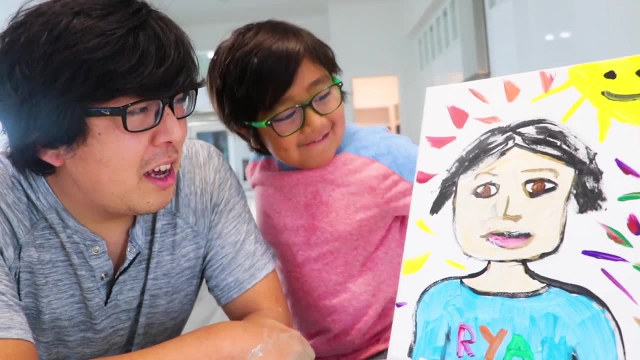 Oh, okay, Oh, I see, Hmm, interesting. You have a drawing style too. I think you got the influence from Van Gogh, Hmm, And Mommy's, hmm, I like it too. There's one thing missing: What? Ryan's not smiling. 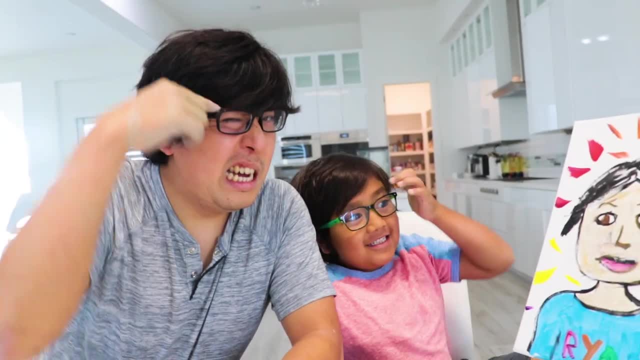 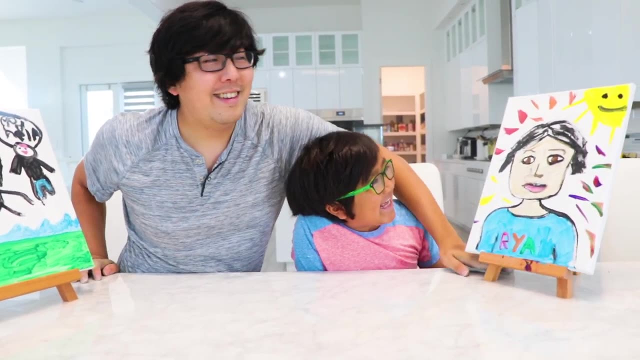 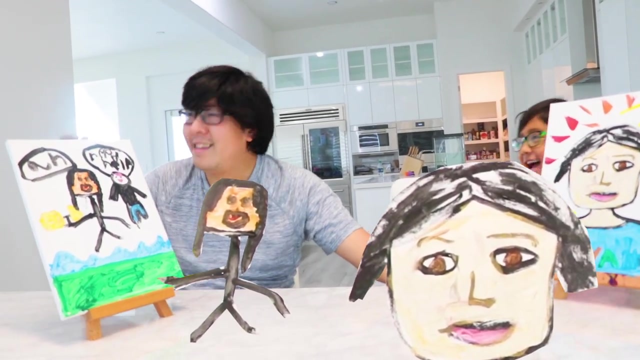 His eyebrows are going mm, mm, mm, Kind of eyebrows. Hey So, but at least the sun isn't smiling, looks like Okay. so which one do you like better, Daddy? I like this one better. No, 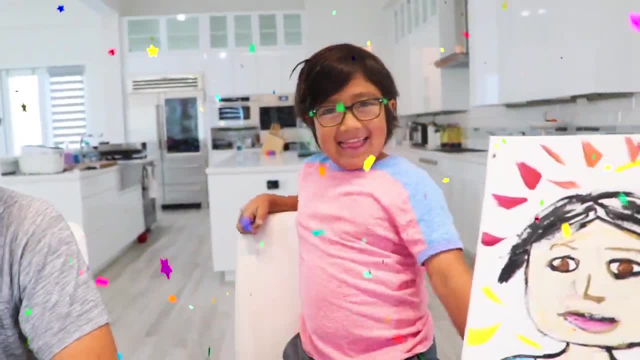 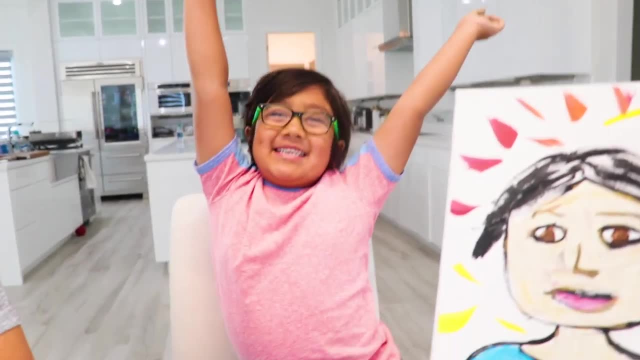 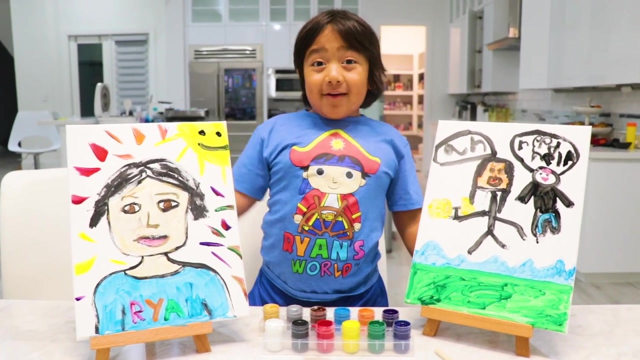 Good job, Ryan. Good job, Ryan. Ryan is the winner of the drawing each other competition. Good job, Ooh, even though I made Mommy a stick figure. Thank you, guys for watching our painting each other video. Bye, Remember, always stay happy and rise. 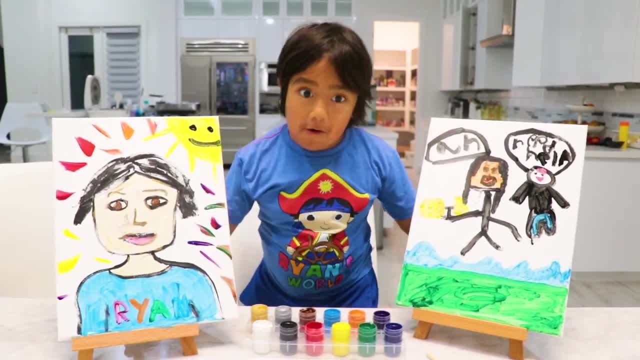 up. Bye Wait, which one's the real, Ryan?